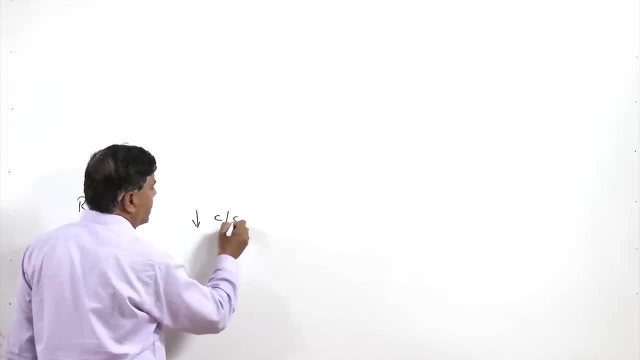 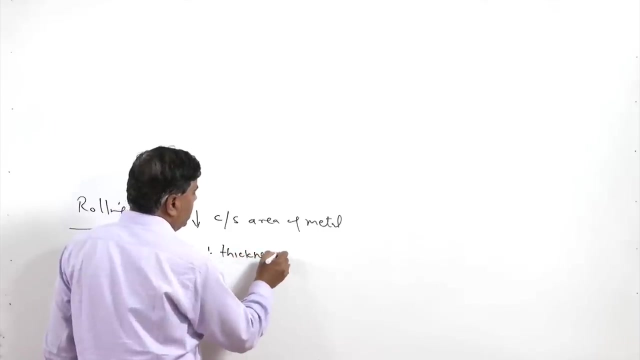 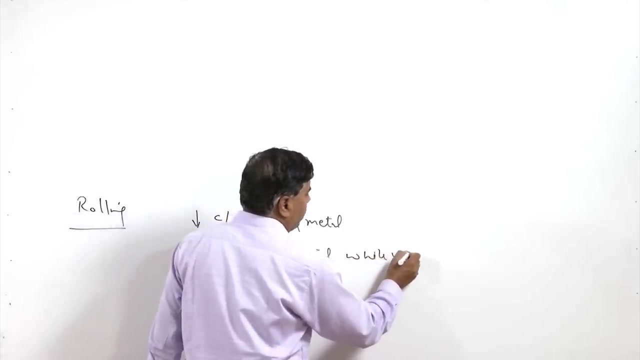 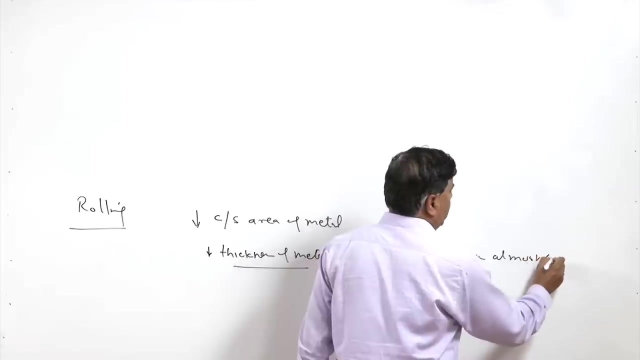 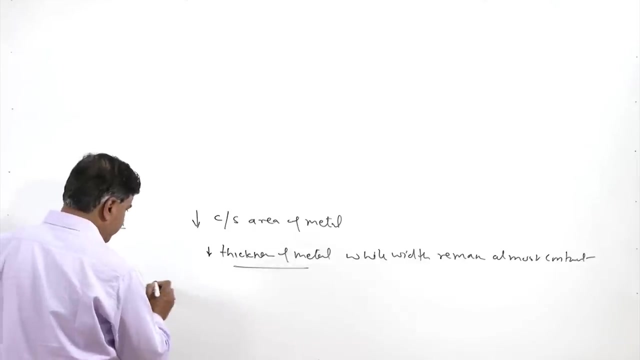 used for the reducing the cross sectional area of the metal stock. So this cross sectional area is used by decreasing the thickness of the metal, So while width remains almost constant. So if, like say, if we see this is the plate before the rolling, then after the rolling its thickness is reduced significantly, like 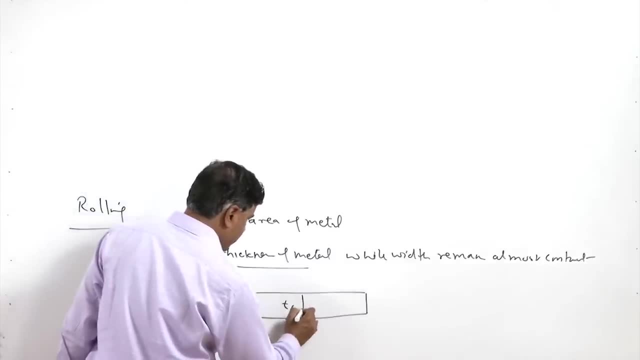 T 0 and T f, like this: T 0 and T f. So T 0 is the initial plate and T f is the final plate thickness which is achieved after the rolling. So whenever this is carried out, there is no change. W almost remains constant. So V 0 and V f. in both the cases it remains. 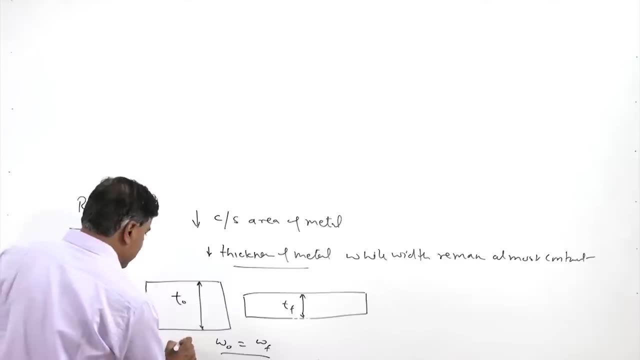 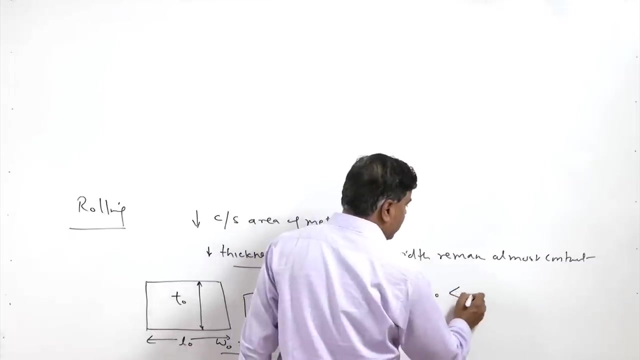 constant, but there is a significant increase in length. So these three components will be forming the volume of the metal. So L 0 is the initial length and L f, which will be significantly greater. So whenever rolling is carried out, what we will see, L 0 is less than the L f and T 0. 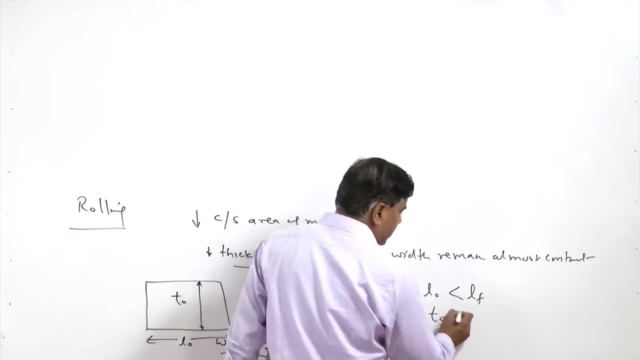 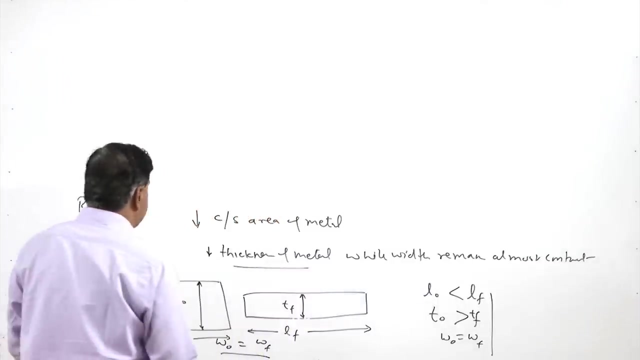 is significantly greater than the T f, So thickness is reduced and length is increased, while width almost remains constant: W 0 and W f. So this is what is achieved after the rolling, How it is achieved through the rolling. that is what we will try to see Whenever. 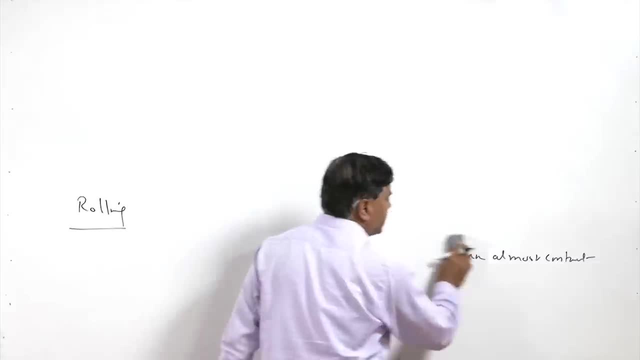 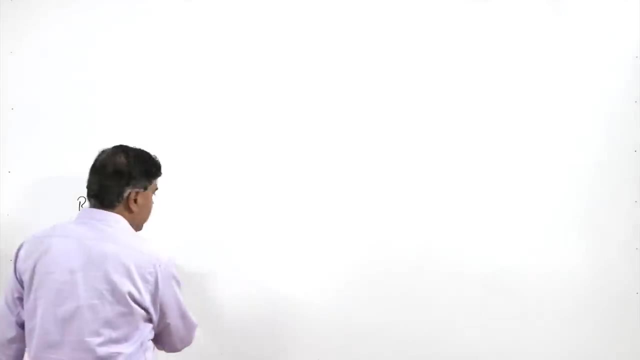 the rolling is carried out, it helps to reduce the cross section throughout its length. The variation in cross section is not possible in case of the rolling and whatever is the length of the product being made through the rolling, it has uniform cross section. So if we consider the case, there are variety of the shapes which can be produced by the 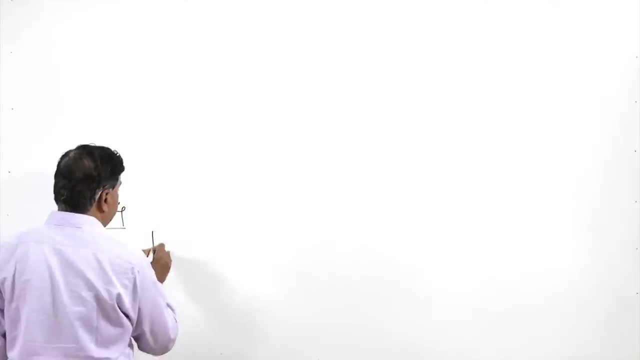 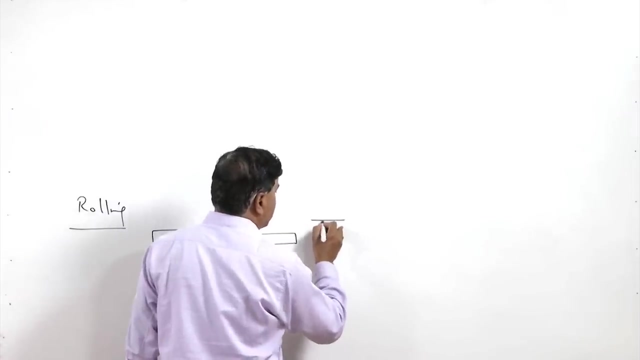 rolling, and these are. these may be in form of, like, say, a square section, in form of the plates, in form of the T section, like this, in form of I section, in form of T section, like this: 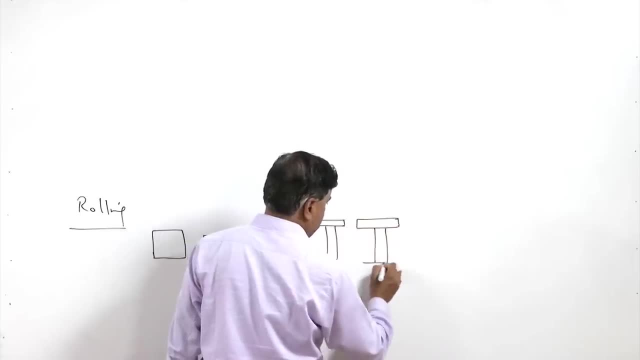 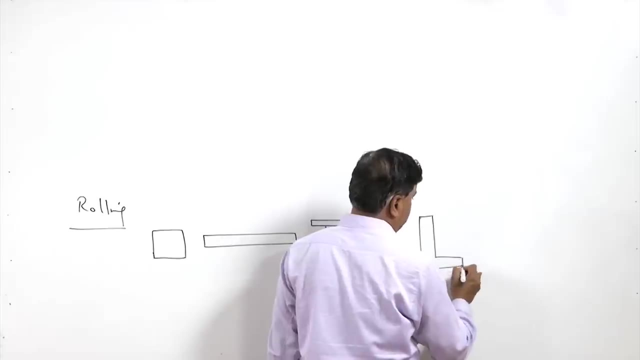 G, n, section L, section C sections, So such kind of numerous simple shapes, oval shape section can be. 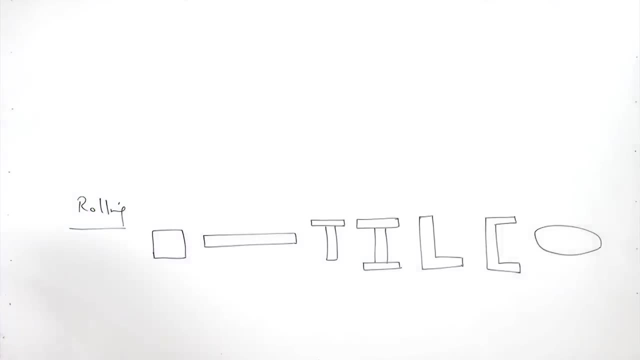 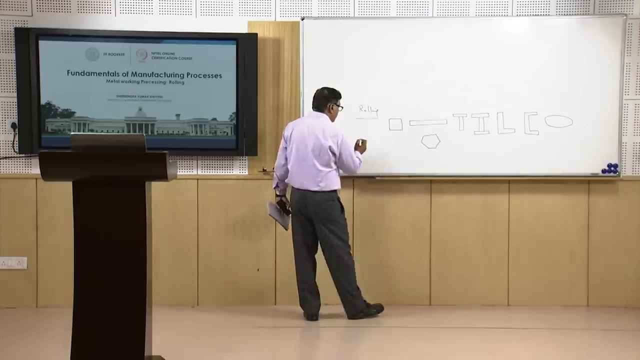 produced easily using the rolling based processes. Otherwise, there are so many other shapes, like hexagonal shape. So all these cross sections, these are the various cross sections of the plate which can be cross sections of the members or stocks which can be obtained. while these sections 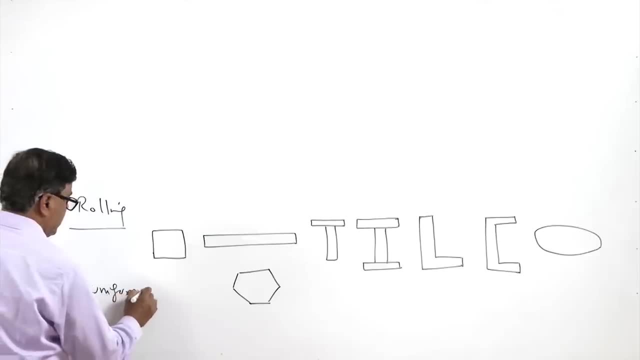 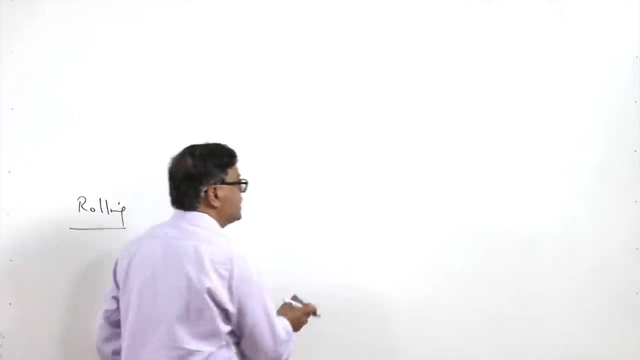 will be uniform along the length. So the variation in cross section is not possible in the products, which is achieved through the rolling. So how it is achieved through the rolling, that is what we will try to analyze. For this purpose, basically, the rollers are used. 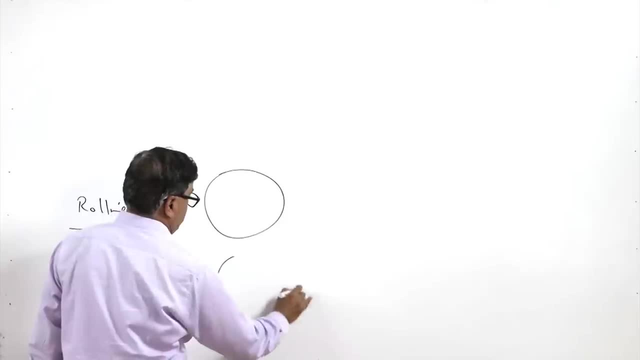 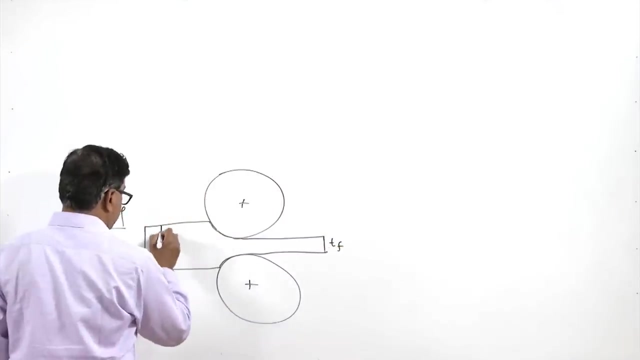 So we can see the rollers in this way: Say, these are the two rollers And this is the plate which is being passed through the rollers, and here it will be reducing the cross sectional area gradually and then it will be passing out this manner. So here this will be the final thickness and this is the initial thickness. T0 and Tf is 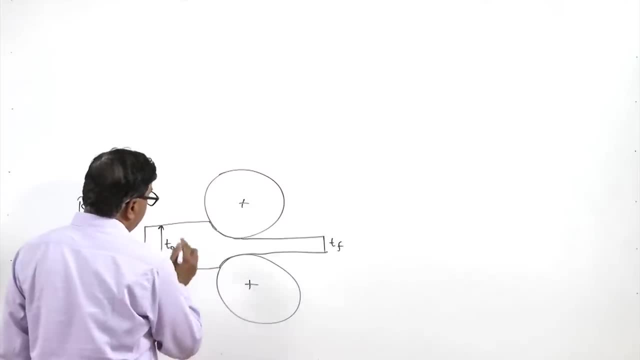 the final thickness, Since if we take any particular length, unit length and width, since whatever reduction is obtained, that reduction happens in case of the thickness only, while the width of the plate, which will be along this, along the, if we can see the same thing in the top view. 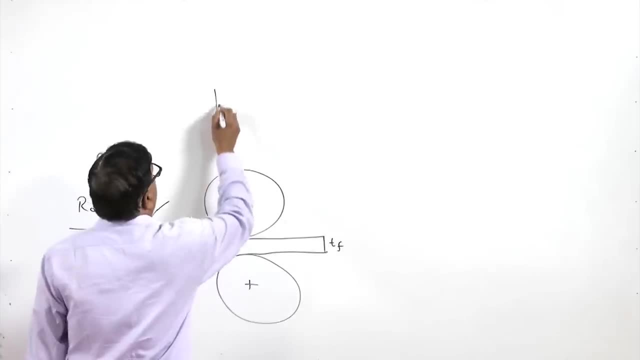 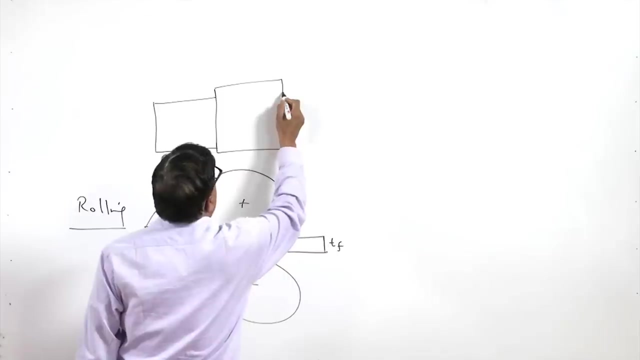 also wherein we can have the rollers in this manner. So this is the thickness, So this is the thickness, And say, the plate entering in the roller, like this, and then coming out in the same width, like this. So this is the axis of the roller. 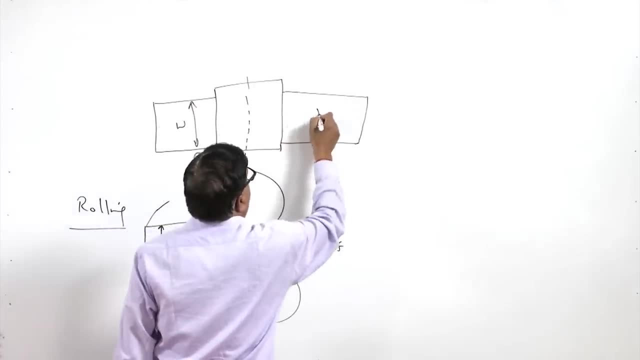 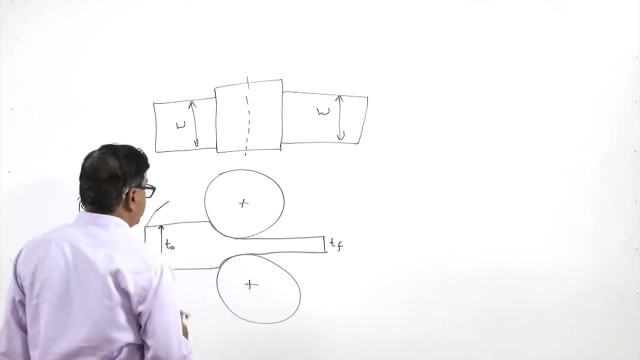 So width of the plate before rolling and width of the plate after the rolling: both are same, but there is a significant reduction. So width is same, thickness is getting reduced. So, considering the constancy of the volume, so what we will be having. 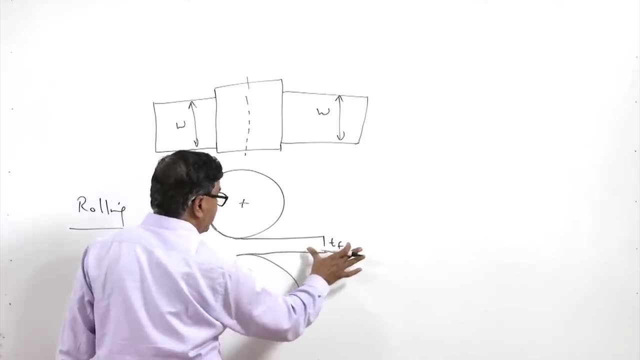 Here for unit length, we will be getting the much greater length of the metal. So the length will be more, thickness will be less and widths are same, which is achieved. So if we consider this is the centre of the roller. So if we consider this is the centre of the roller, 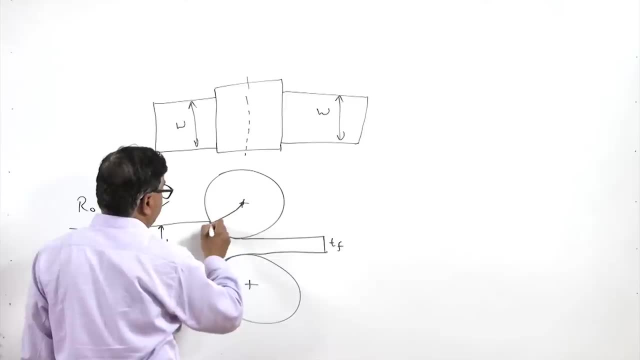 Centre of the roller And width And width. This is the radius R of the roller and this is where the plate is coming out of the rollers. So entry is taking place at this point and exit is taking place at this point. So this is the entry point and this is the exit point. 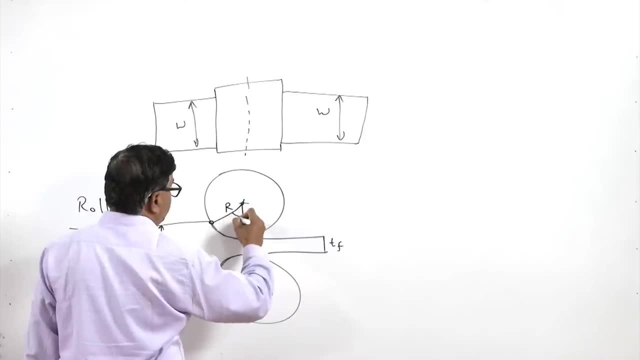 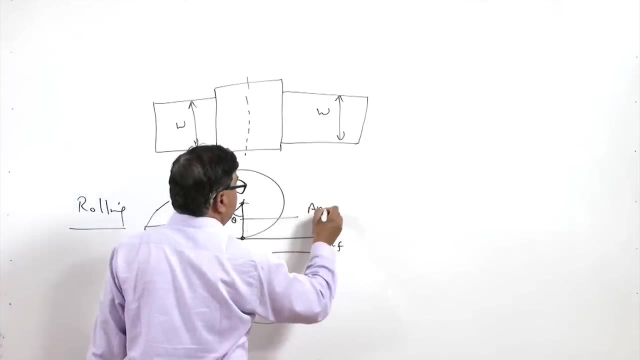 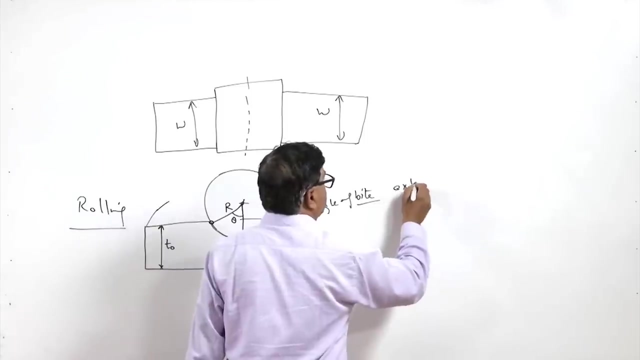 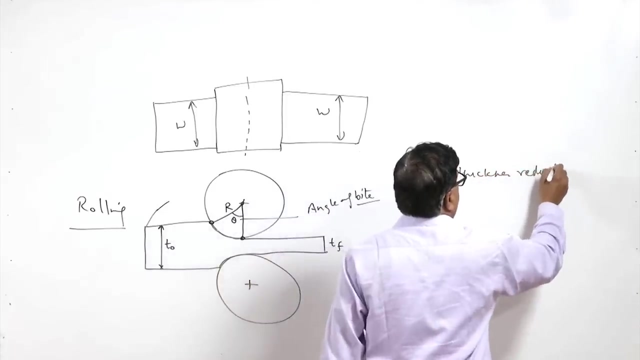 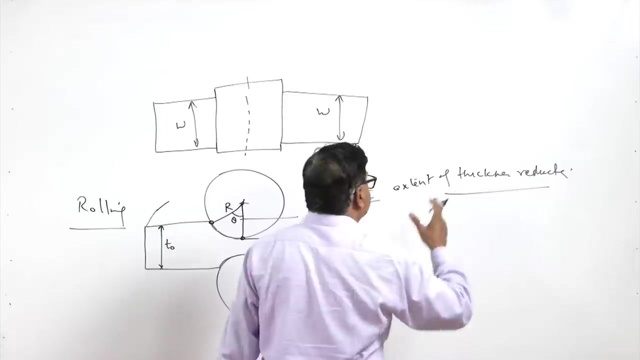 And angle formed between these two points is called theta and which is basically the angle of bite. It determines the extent of thickness reduction which will be taking place. So greater the extent of the reduction in thickness, greater will be the draught which will be achieved during the rolling 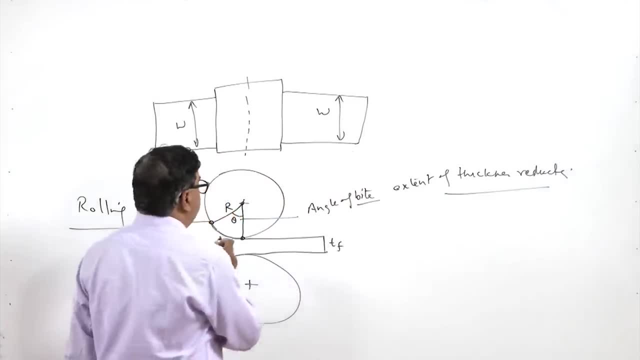 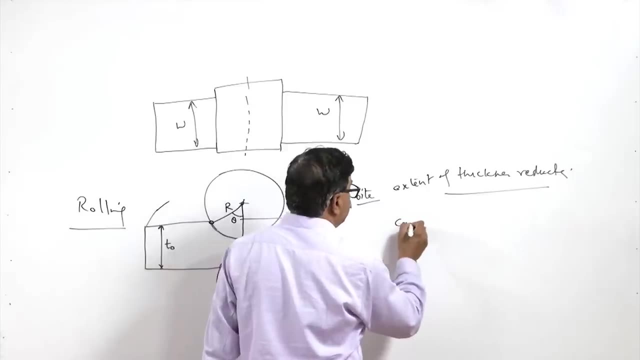 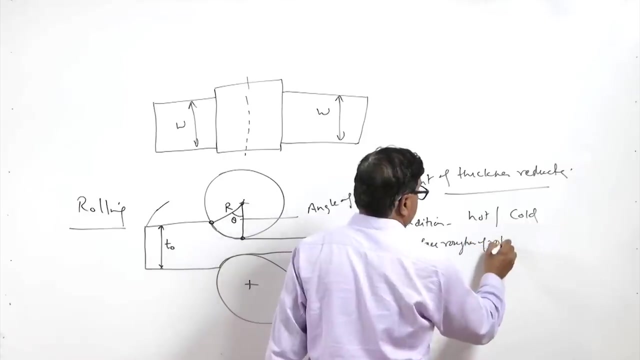 So this is the angle of bite. So this angle of the bite also depends upon the condition in which the rolling is being carried out. means it is hot or it is cold, or the surface roughness of the rollers. So for smoother surface or for smoother surface, 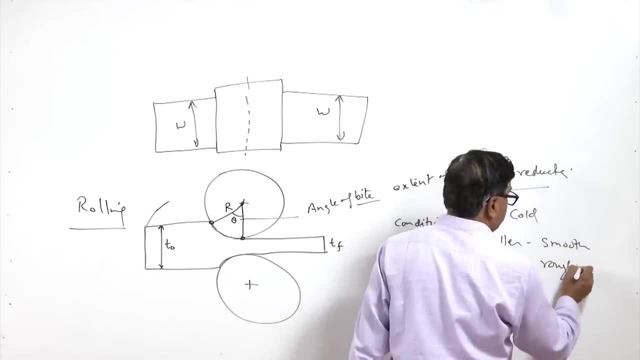 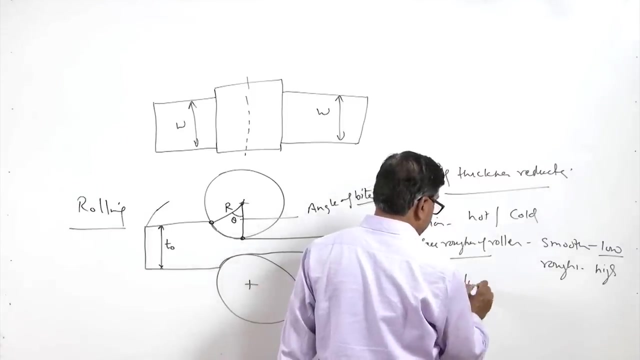 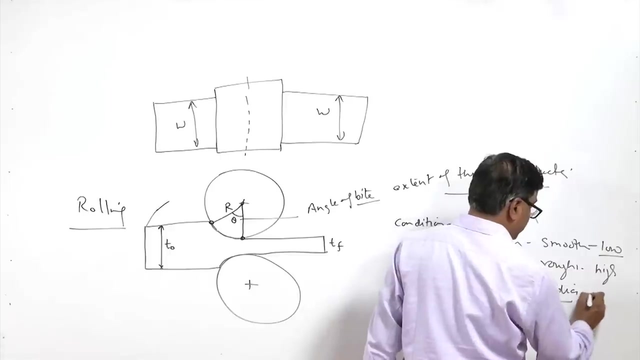 Okay, So for smoother surface or for rough surface? So for smooth surface, low angle of the bite is used, while for the rough surface high angle of the bite is used. The diameter of the rollers: large diameter of the large dia rollers used for the low. 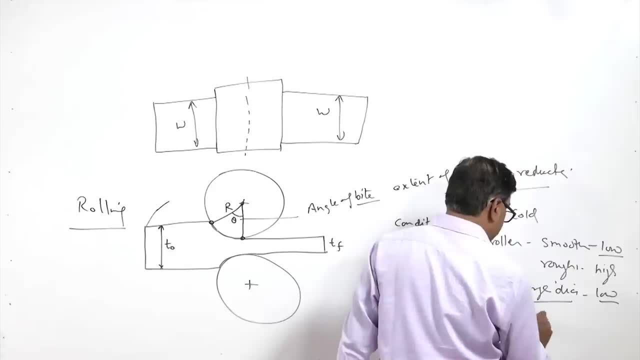 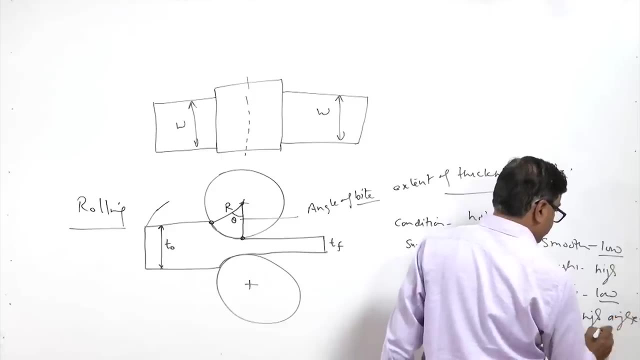 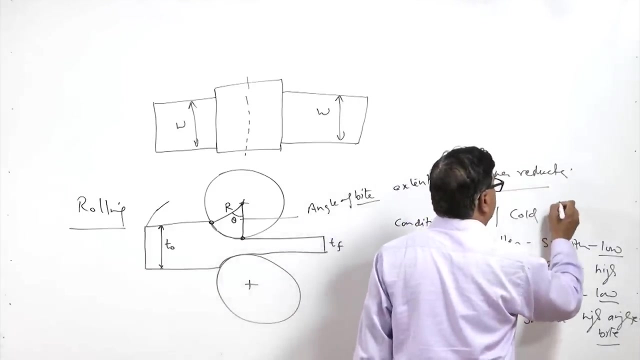 angle of the bite, While the small dia rollers result in the rough surface. Okay, So this is the angle of the bite. So this is the angle of the bite. So this is the high angle of bite. So the hot and cold rolling angle of the bite. for cold it is very low, like 3 to 4 degree. 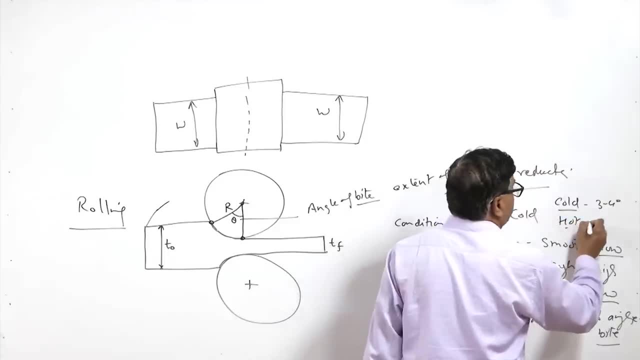 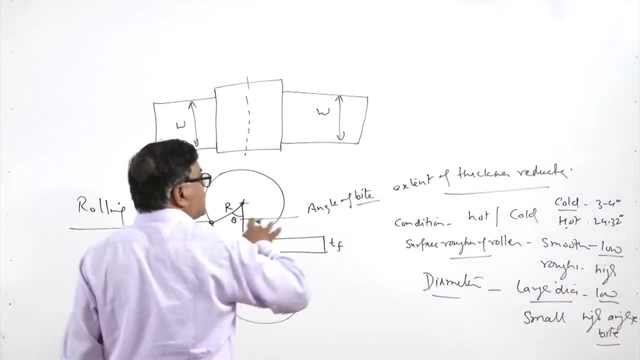 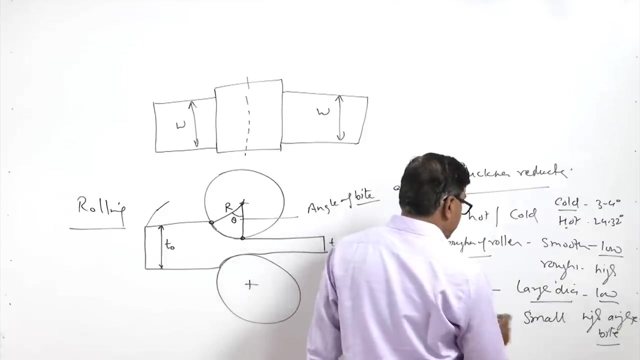 but for the hot it is very high, maybe like 24 to 32 degrees also. So, since the angle of bite determines that, Okay, So this is the angle of the bite. So this is the angle of the bite, This is the extent of reduction, which in turn, is influenced by the diameter of the rollers. 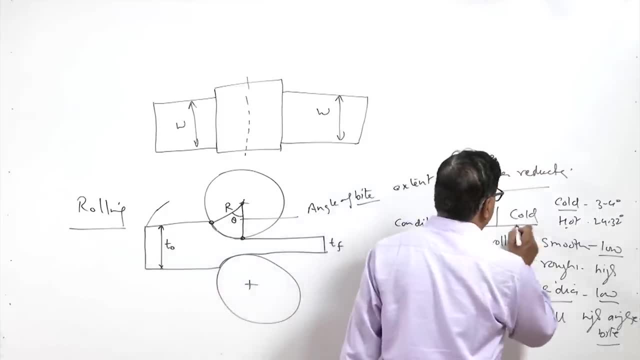 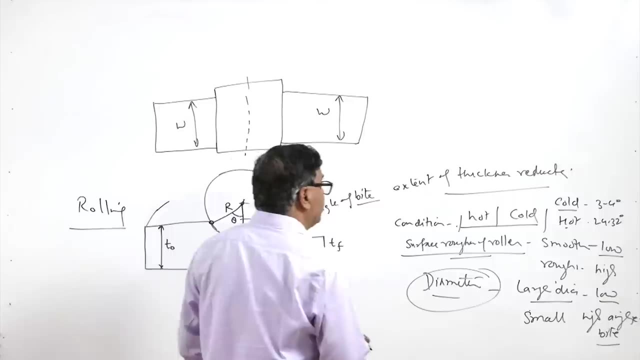 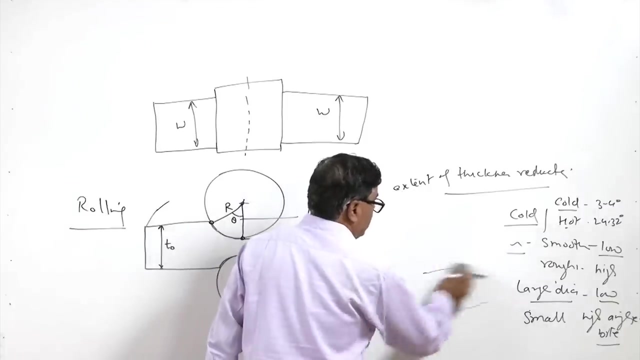 surface roughness of the rollers and the condition or the temperature of the metal in which rolling is being carried out. So, with regard to that, if we see, these are the factors which will be governing the angle of the bite which can be used, which eventually be determining the extent of the rolling. 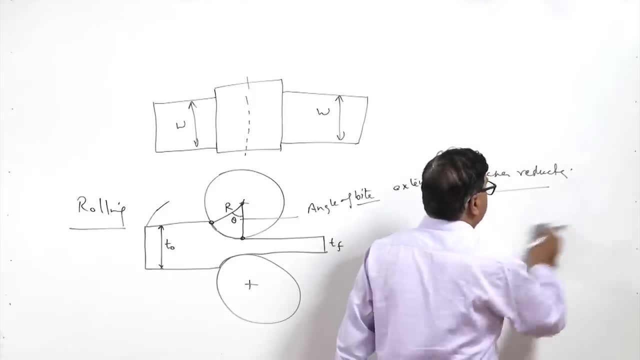 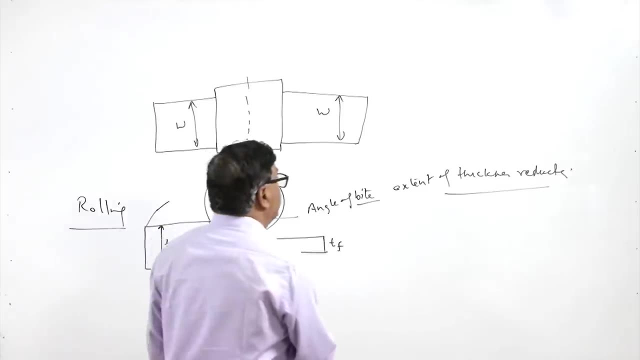 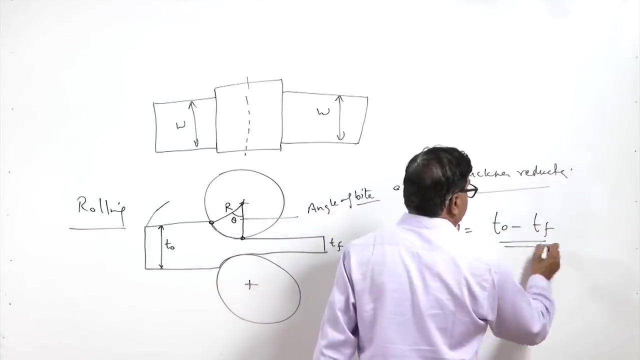 Okay, So this is the extent of the reduction during the rolling. So this is what is defined as a draft Draft. D is basically the difference in the initial plate thickness to the final plate thickness, So the maximum draft which can be achieved. Okay, 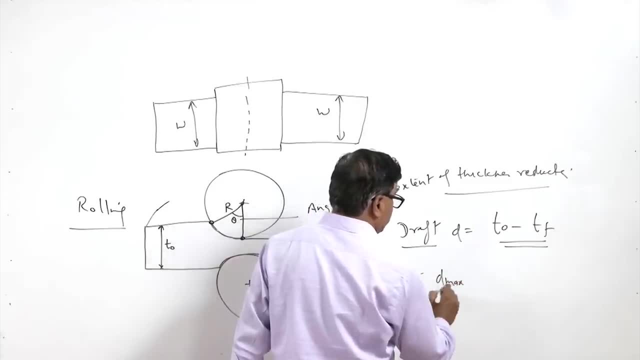 So the maximum draft D max which can be achieved is found: a function of the mu square into r, wherein mu is the coefficient of the friction, coefficient of friction between the metal and the rollers. So if the surface roughness is more, If the surface roughness is more, 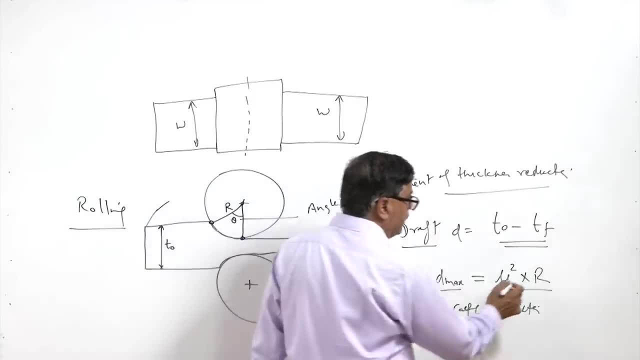 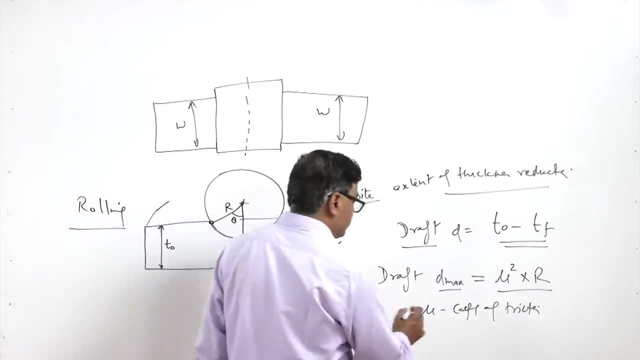 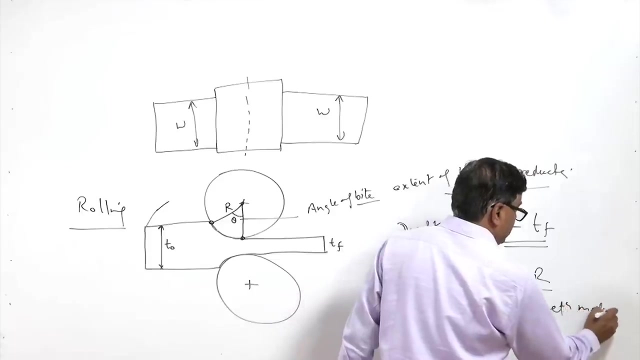 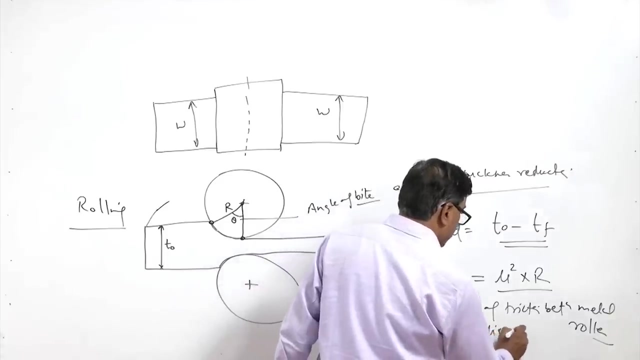 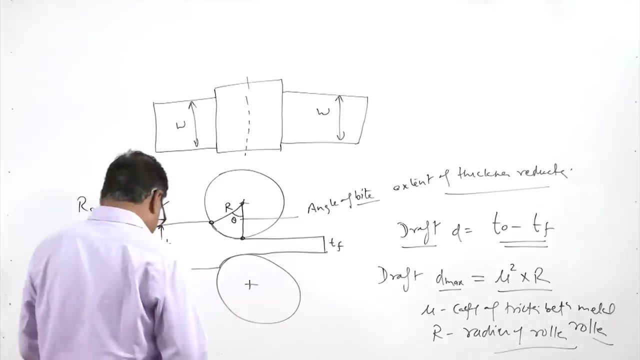 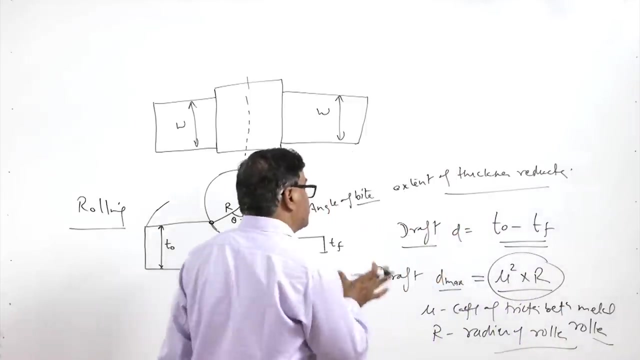 The draft, more draft is possible. and if the roller diameter is more than, the more draft is possible. So the friction coefficient between the metal and the roller surface, and r is the radius of the roller which is being used for the rolling purpose. So this will help us to determine what is the maximum extent of the draft which can. 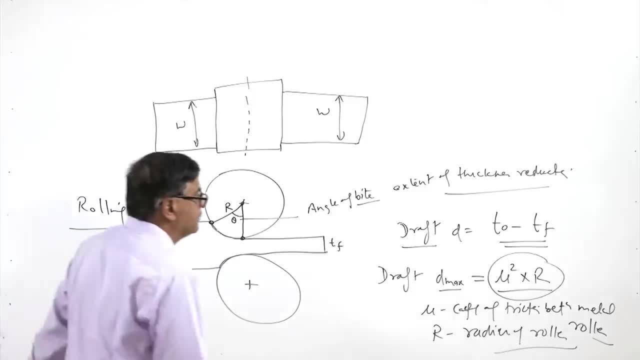 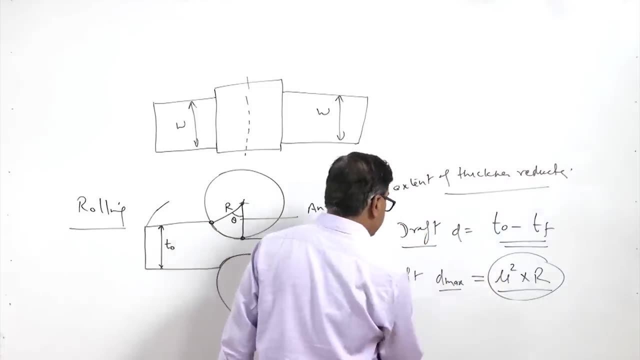 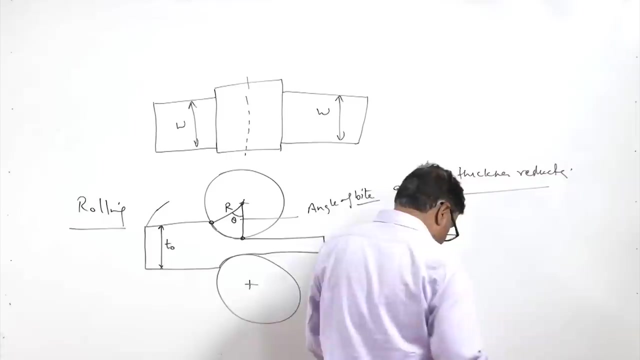 be achieved during the rolling. We know that at the high temperature, at high temperature, the coefficient of the friction increases, which helps in increasing the draft. So if we see, with regard to that, The coefficient of friction mu is found 0.1 for cold working mu is in the range of the 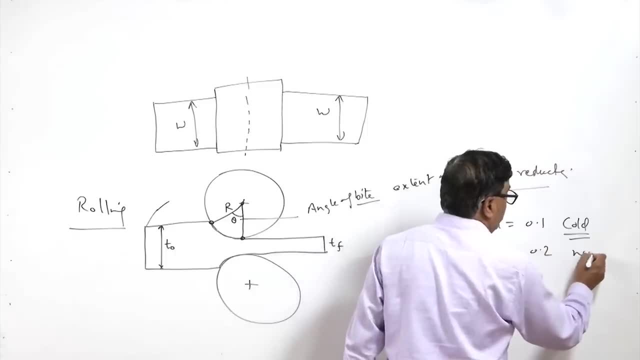 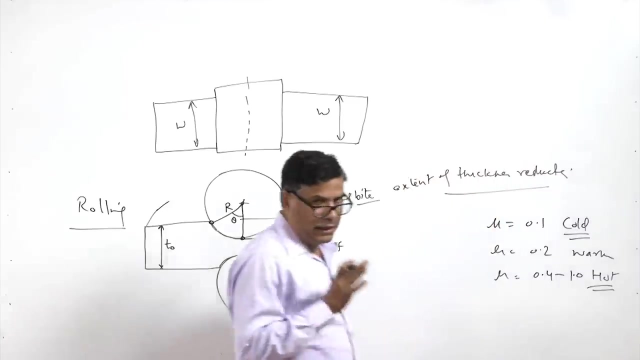 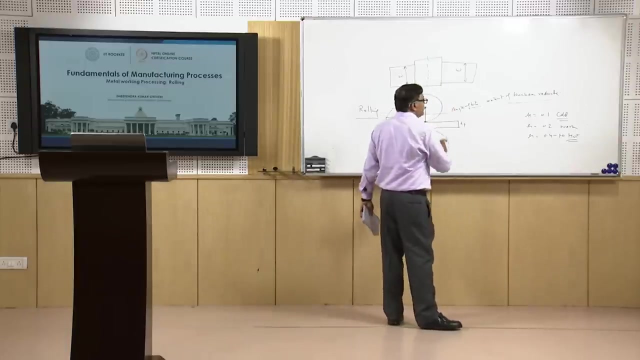 point is 0.2 for warm working and mu is 0.4 to 1.0 for hot working conditions, because at the high temperature The metal gets a softened and it forms more grip with between the matting surfaces, which in turn increases the friction coefficient. 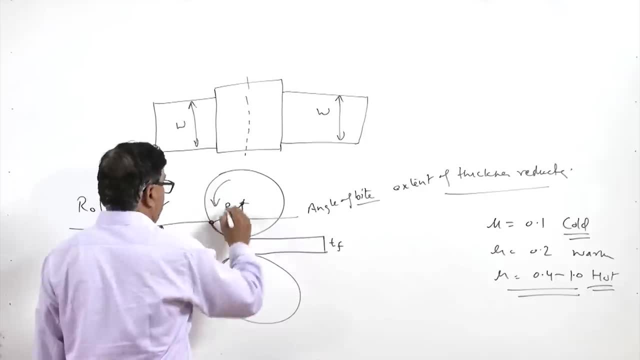 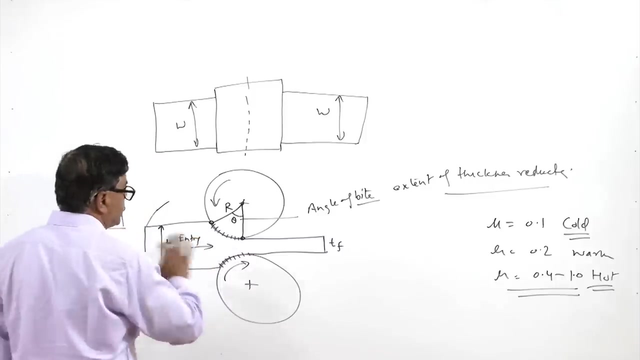 So basically during the rolling, when the rollers are rotating, So the friction between the roller and the plate surface actually tends to pull it in between the rollers. So when the metal enters in the rollers, This is where entry of the metal takes between the rollers. 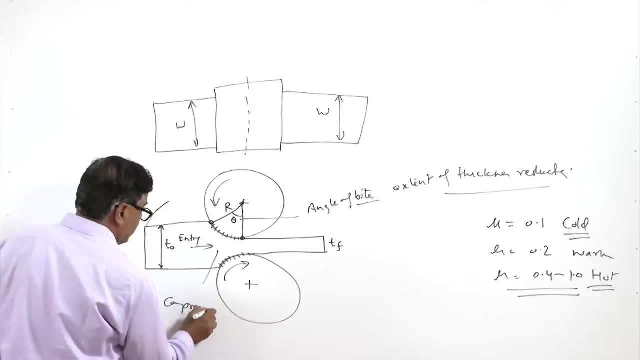 So here it is compressed, and compression leads to the reduction in the thickness of the metal by deforming it plastically. So here the metal may have the equiaxed grain, but when it is deformed plastically after passing through the rollers, Here it will be elongated. 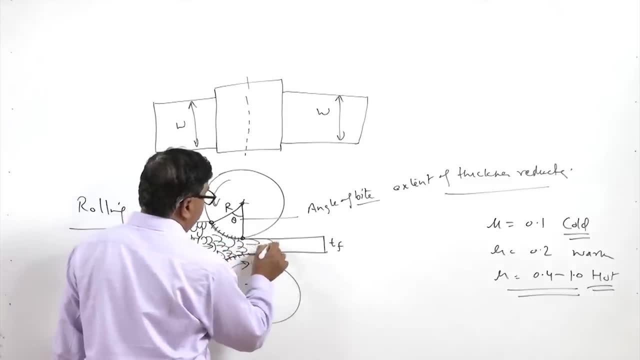 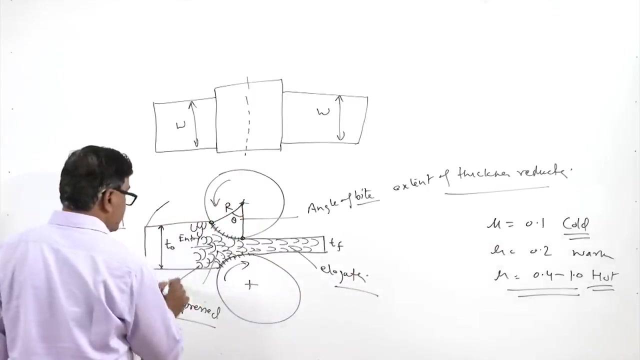 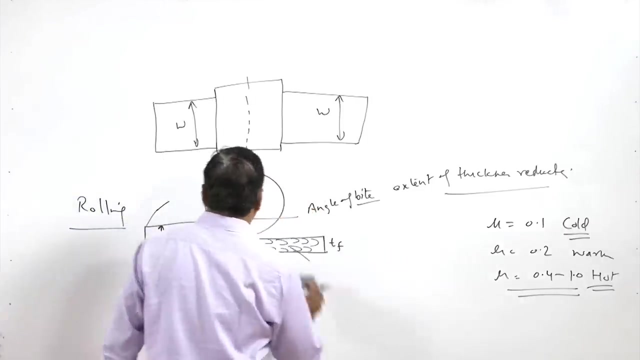 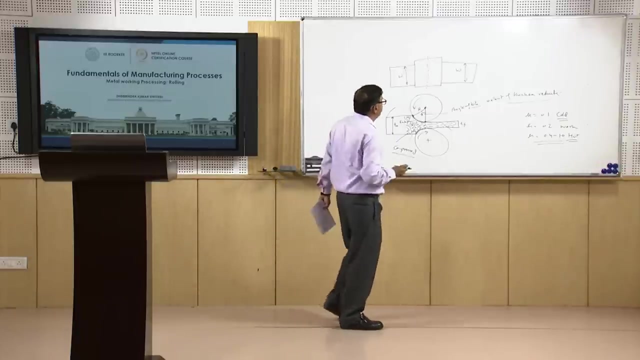 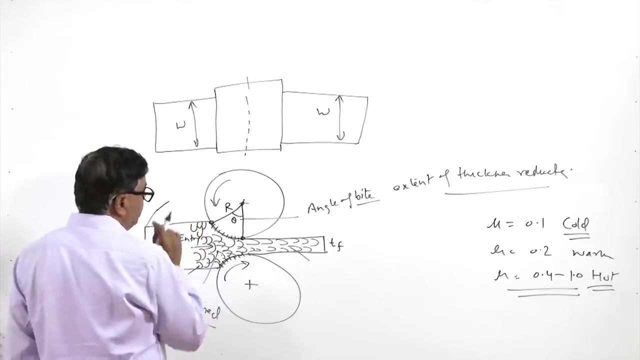 So after the deformation it gets elongated significantly like this. So the elongation after the deformation and equiaxed grain before deformation is found. So this is the case when the two rollers are being used. So when the material is deformed by the rolling we will see that the metal entry, the speed, 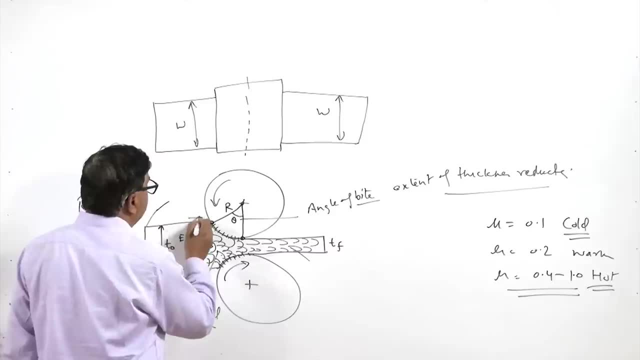 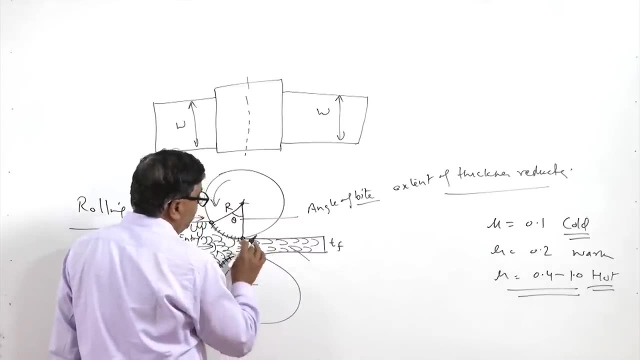 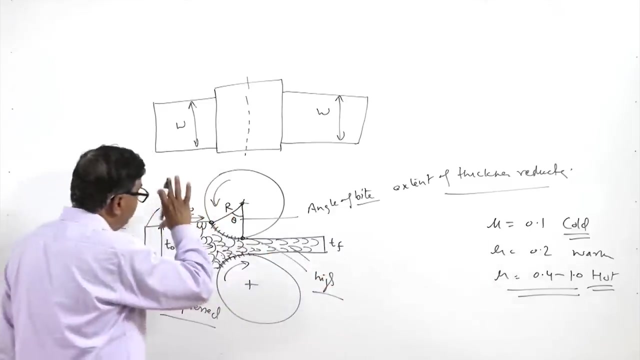 of the metal at the time of entry between the rollers is very low, and the speed of the metal between the rollers when at the time when it comes out is high. So at the exit the speed is high. Well, So the speed is low. 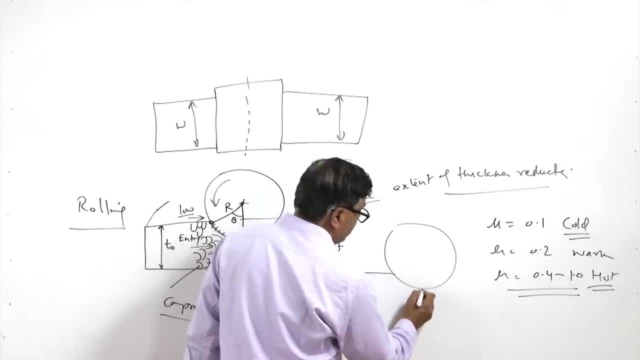 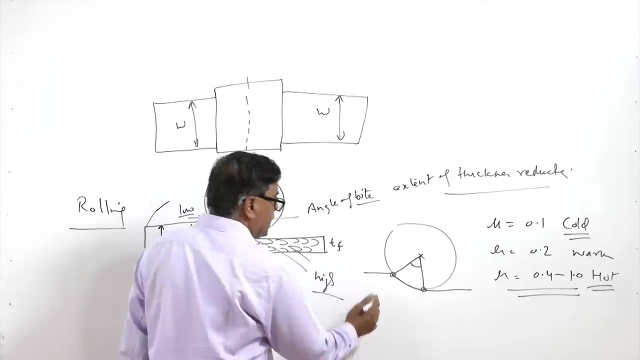 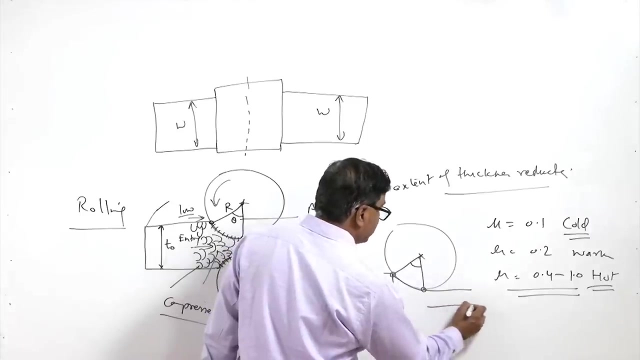 So if we see in this configuration, here it exits and here it enters, This is the angle of the bight and this is the center. So the speed is low here and speed is high because here the volume of the metal for a given volume of the metal, this is the thickness, and when it comes out the thickness is significantly. 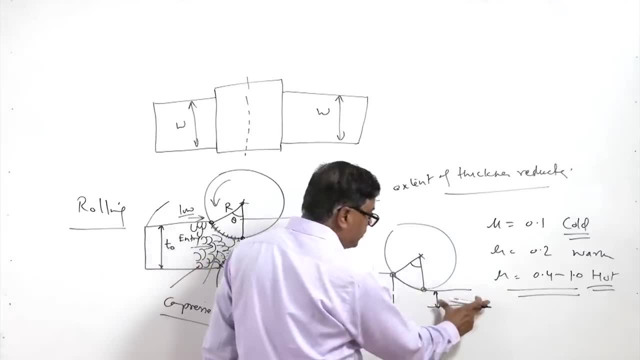 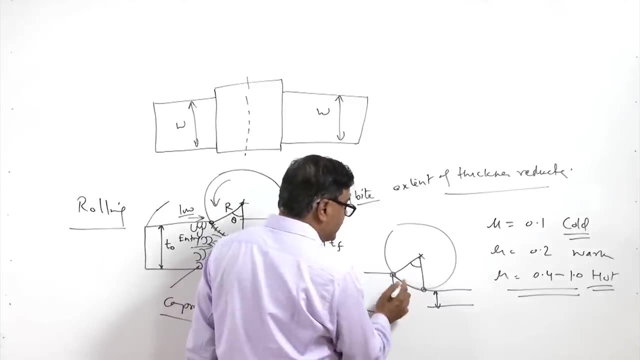 less. So in unit time it comes out with the greater length. so the speed of the metal in the beginning becomes low and it keeps on increasing until it exits. so it comes out of the rollers. So what happens when the metal enters between the rollers? so initially what we see, that 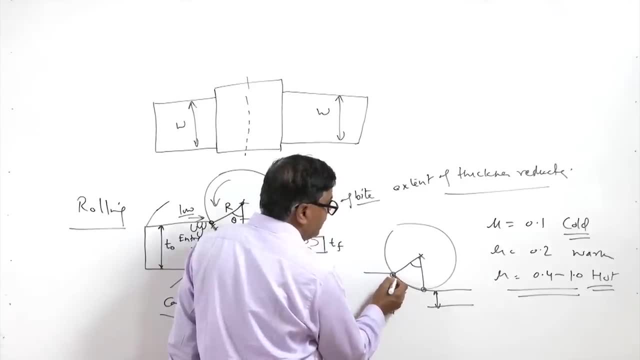 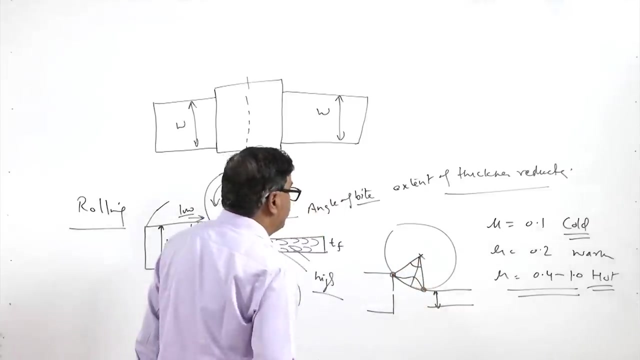 the metal. pressure builds up in the metal and then it will keep on increasing and then again it will keep on decreasing. So maximum pressure is found somewhere at the neutral plane here. So what is this neutral plane? so what? we see that the roller is rotating at the certain 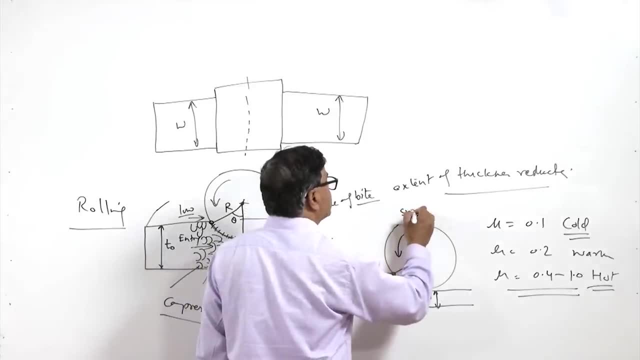 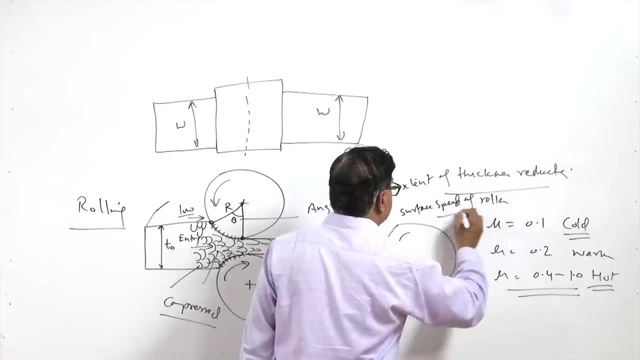 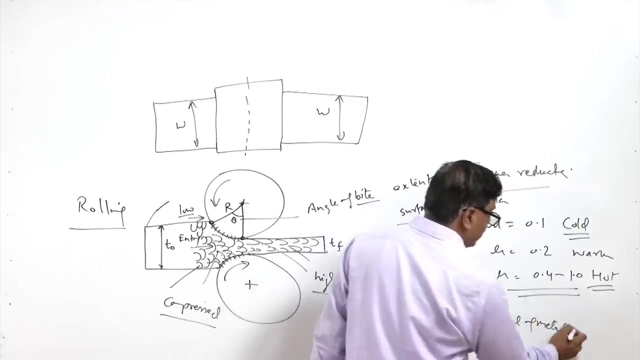 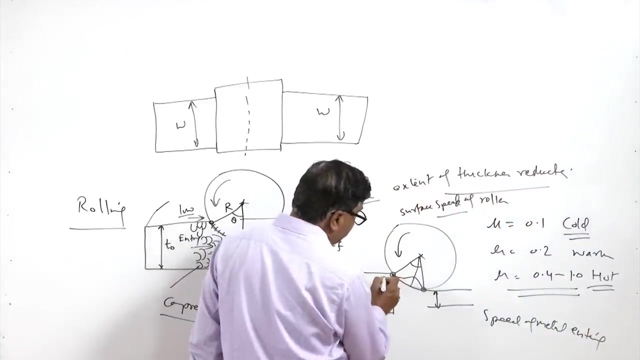 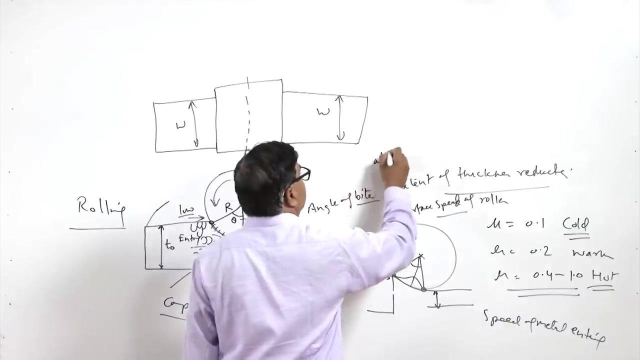 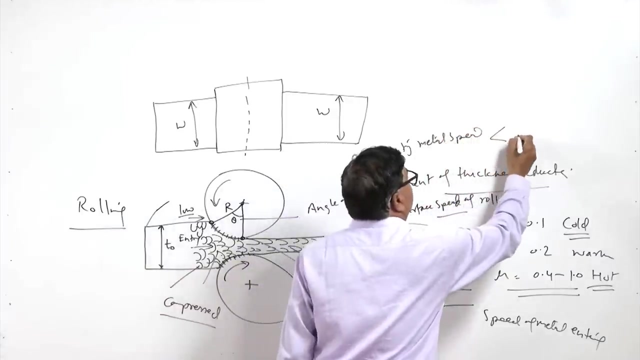 speed. so there is surface speed of the speed of roller and there is some speed of the speed of the metal which is entering, entering. So in the beginning the metal enters, speed of the metal entering is low, while the speed of the roller is high at the entry point. so at entry the metal speed is less and roller 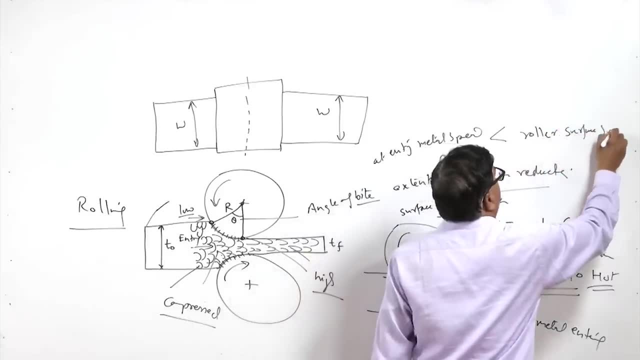 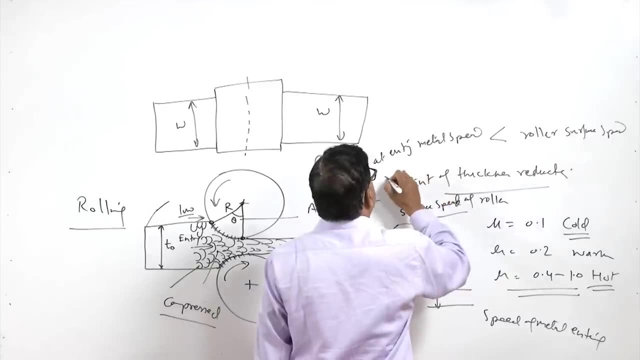 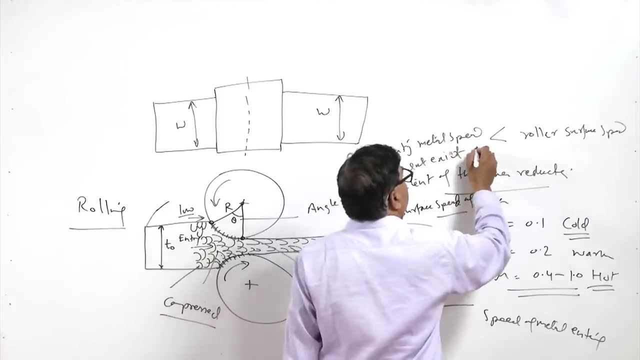 surface speed is less, So at the entry point. So at the entry point. So the speed of the roller is high. This while at the end the reverse happens: the metal at exit, metal speed at exit is higher than the roller surface speed. 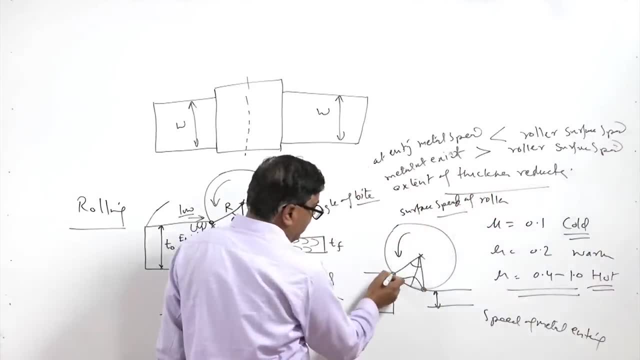 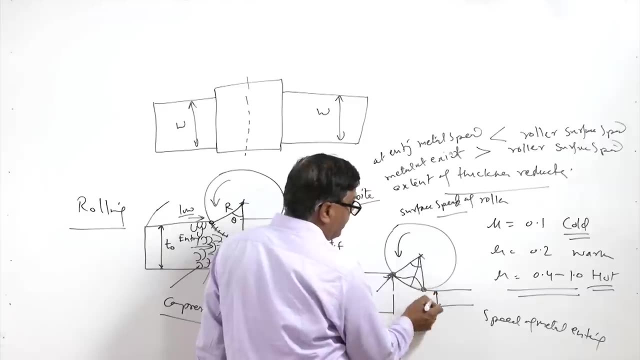 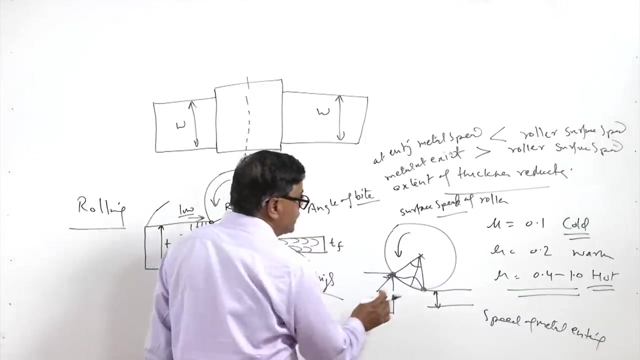 So there are two things. one, when the metal enters, the speed of the metal with respect to the roller surface is less. When the metal comes out, the speed of the metal with respect to the roller surface is high. In between, somewhere, the speed of the metal which is entering between the rollers and 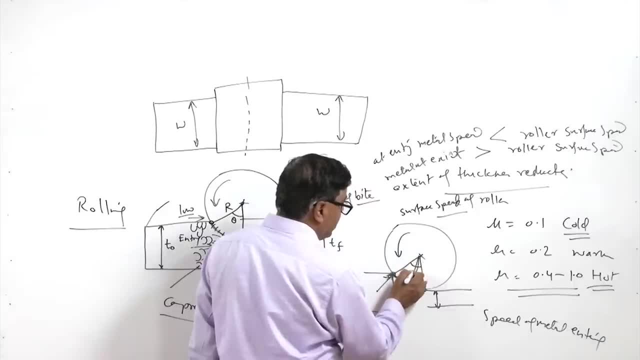 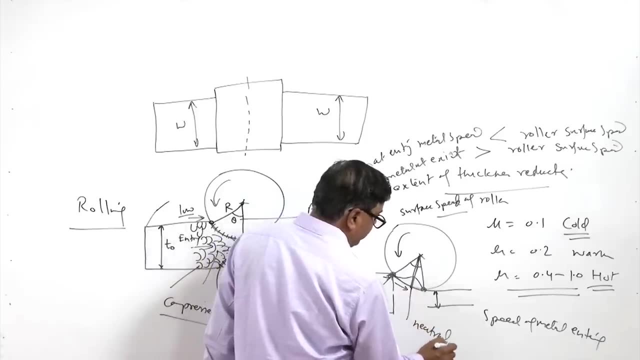 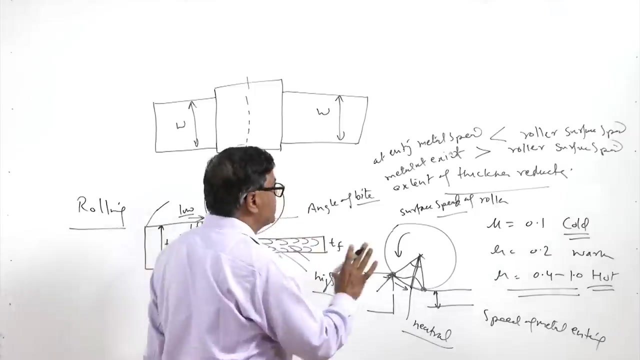 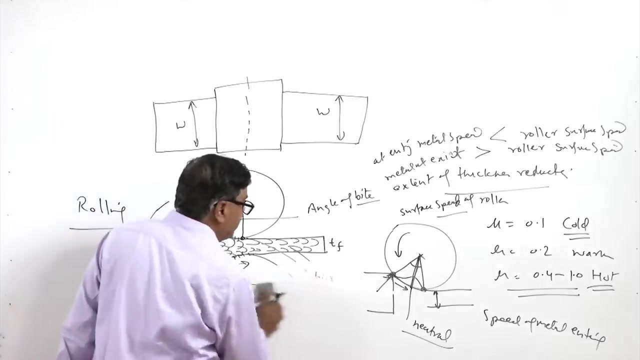 the speed of the roller surface. both are same. so that plane where it happens, that is called neutral plane. At the neutral plane, the speed of the roller surface and the speed of the metal both becomes equal. So if we see, with regard to the way by which pressure builds up during the rolling between, 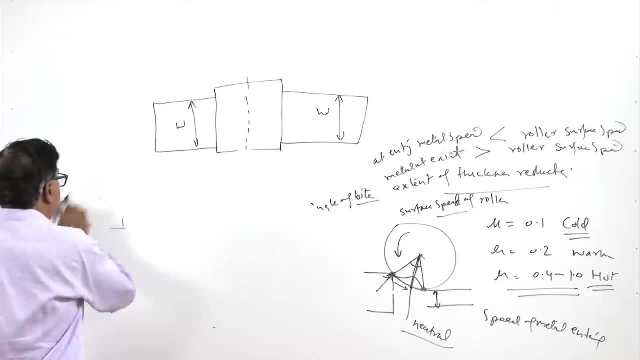 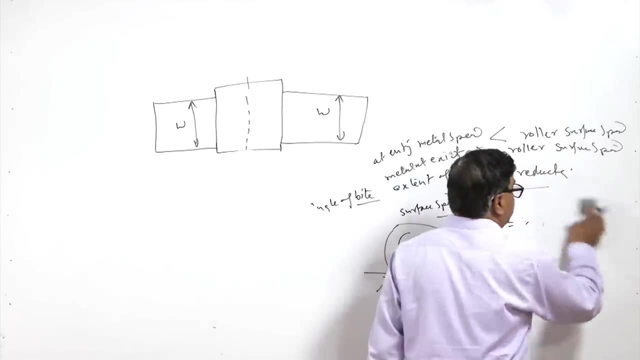 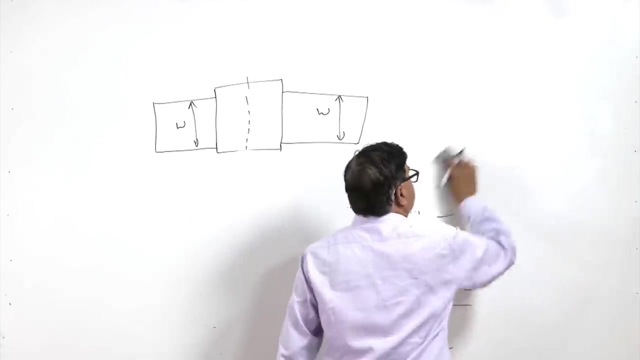 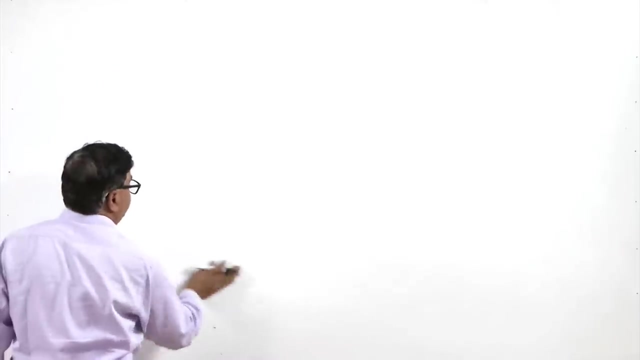 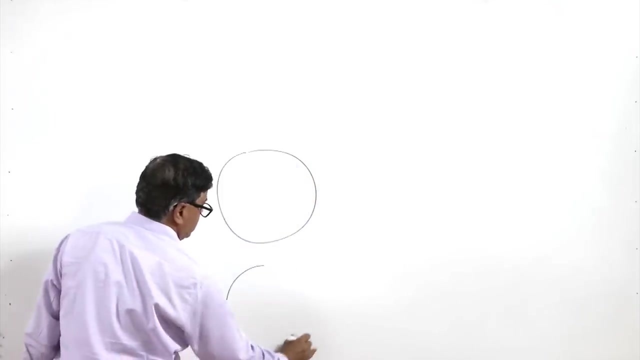 the rollers on to the metal. and how can we calculate the forces acting on to the rollers: torque being consumed, The torque acting on, The pressure acting on and the power being consumed. that is what can be calculated using some fundamental equations. So here, the rollers- center of the rollers, the plate, metal entering. 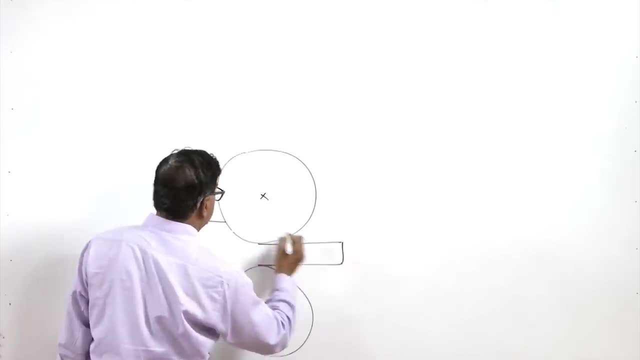 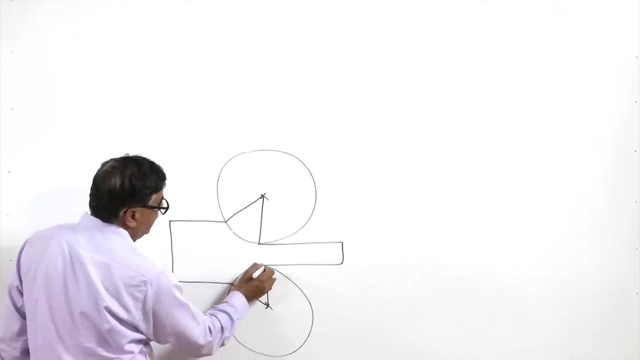 And then it is coming out. this is the angle of the bite. this is the angle of the bite this side. So in both the sides we will see the pressure gradually build up and then it reaches to the maximum level and then it starts decreasing. 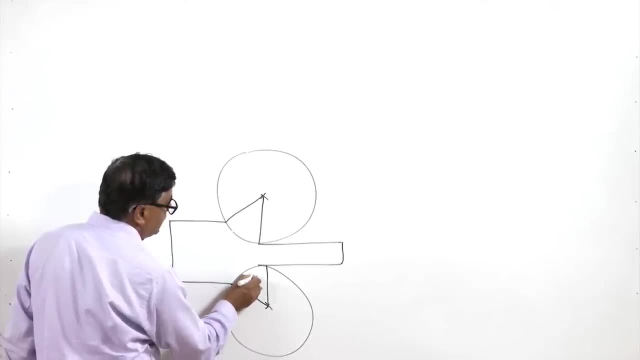 So the variation in the pressure build up is seen like this: where it is maximum somewhere at the neutral plane and then it starts decreasing. at the time when metal comes out of the rollers, it is the pressure is released and the pressure is reduced. and this is the angle of the bite. 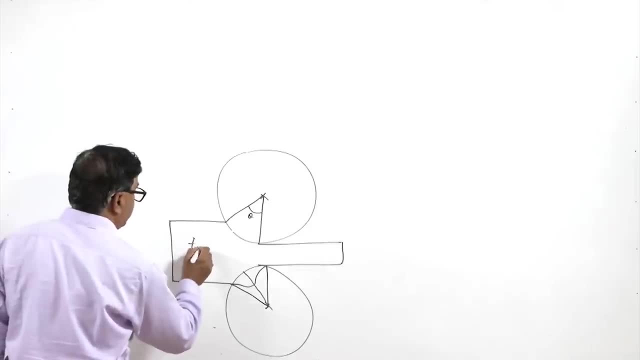 So in this process of the reduction in the thickness- the initial plate thickness and the final plate thickness- this is used for calculating the true strength. So strain on account of the rolling is calculated using the simple equation, the log of T naught. 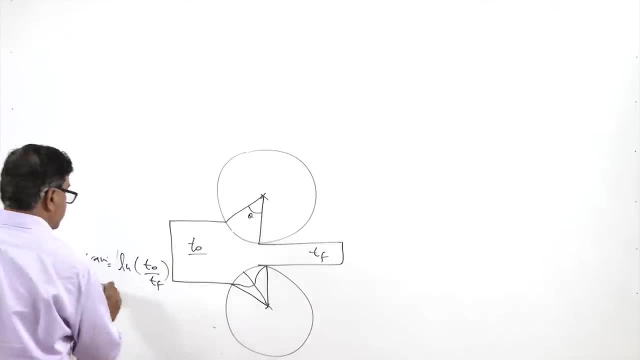 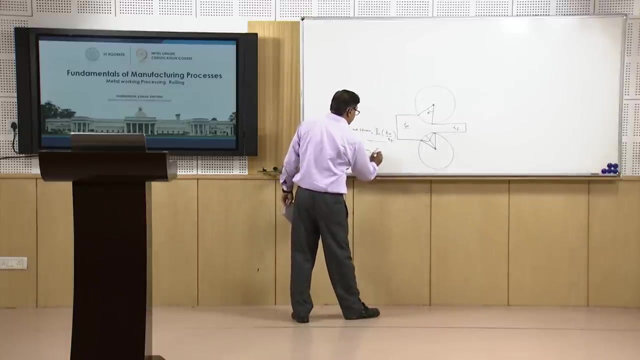 divide by T f. So this is the simple equation for calculating the true strain and then average flow stress. acting flow stress of the metal, under which the metal will be deforming, can be calculated using, like, say, sigma f is the flow stress which can be calculated using the k strength. 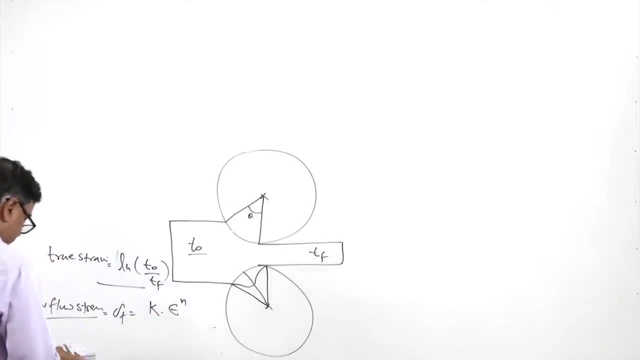 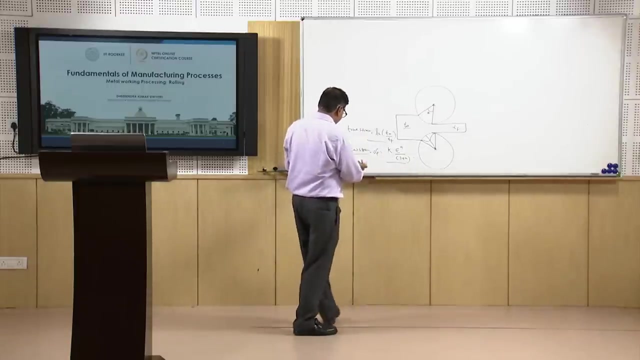 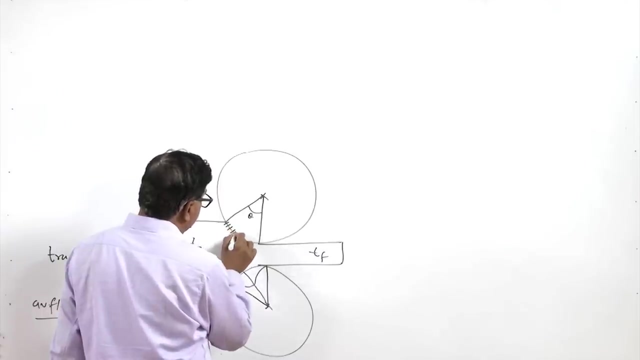 coefficient, strain raise to the power n divide by 1 plus n. n is the strain exponent, and so the k is the strength coefficient. So this is how it, the average flow stress, can be calculated. and if we have to determine the contact length, that is means this length of the contact between the rollers and the 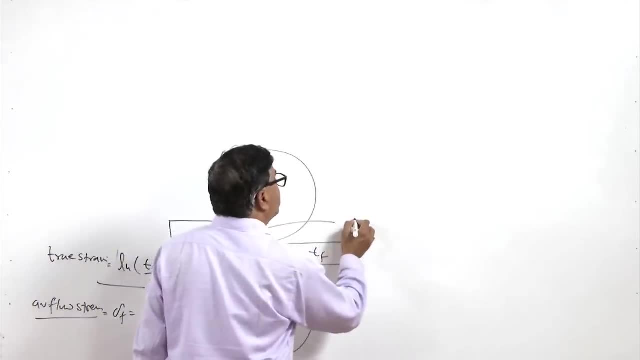 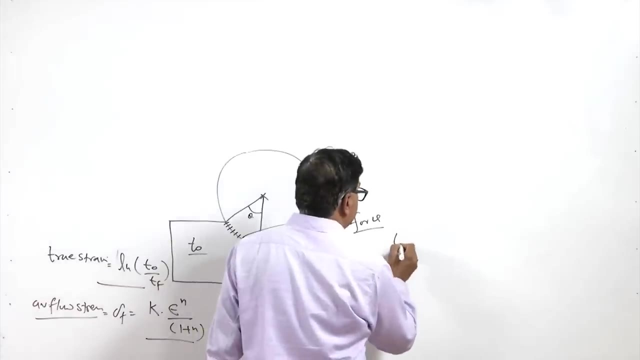 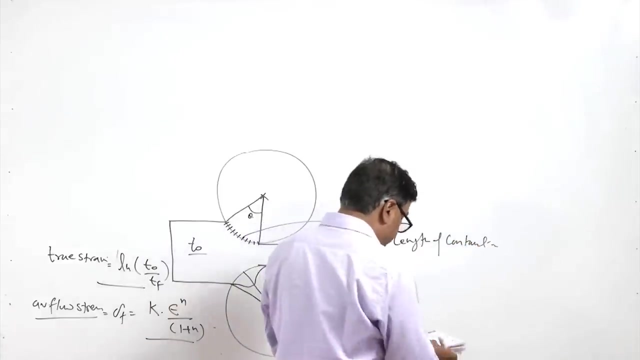 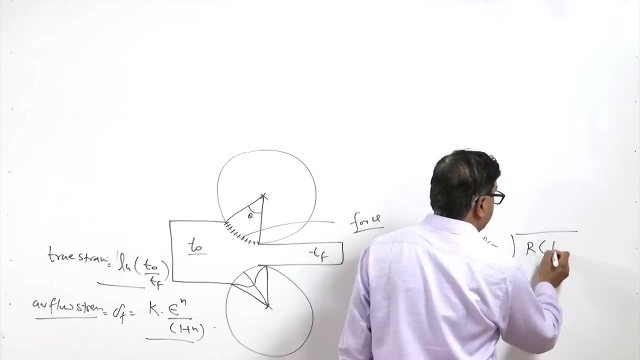 metal which will be governing the force to be applied for the given flow stress. So this, the length of contact, can be obtained using the simple equation: r is the roller radius multiplied by T naught minus T, f. square root of this one can be used for calculating. 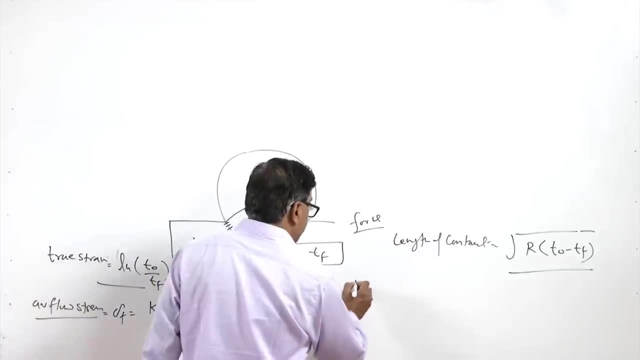 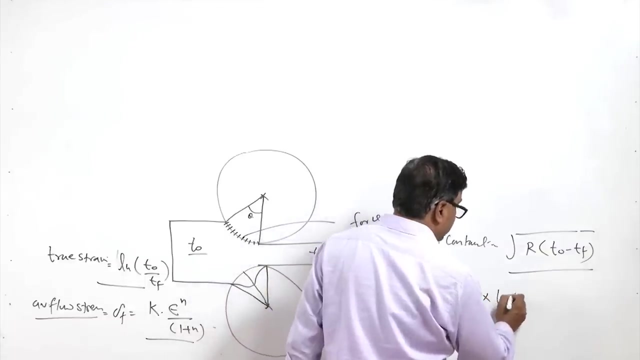 the contact length, Then the roller force or the force acting on to the rollers or the rolling force can be obtained from the product of the flow stress multiplied by the contact length, multiplied by the width of the plate. So L is the contact length and W is the width of the plate which is being rolled, and sigma. 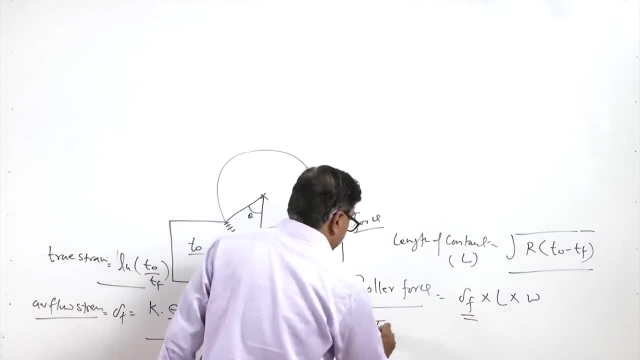 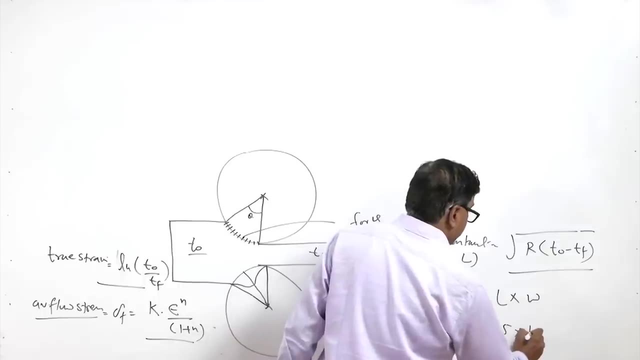 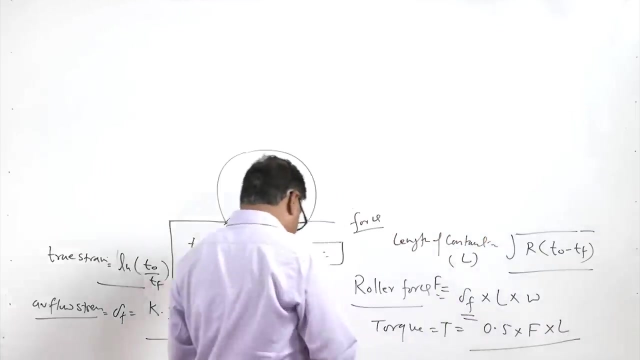 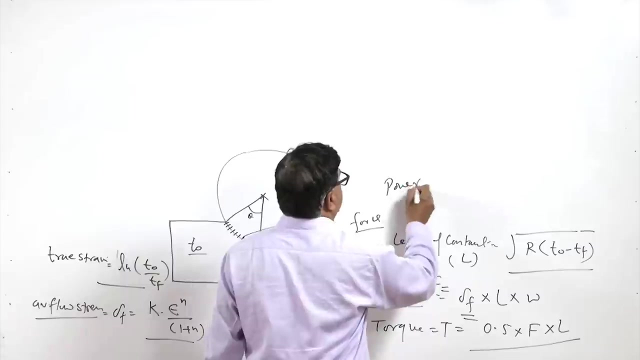 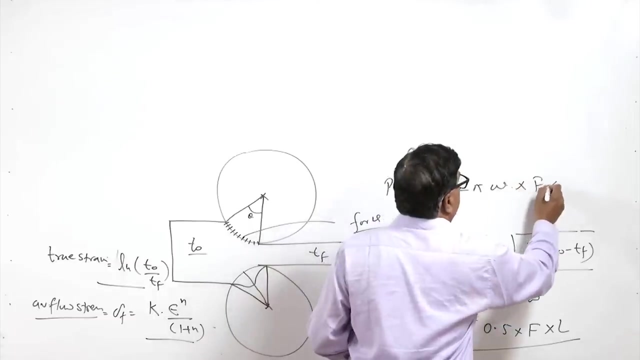 f is the flow stress And the torque can be calculated. T can be calculated using the equation 0.5 times of the rolling force f into the contact length and the power for the rolling can be obtained using the simple equation of the 2 pi mega into the rolling force multiplied by the contact. 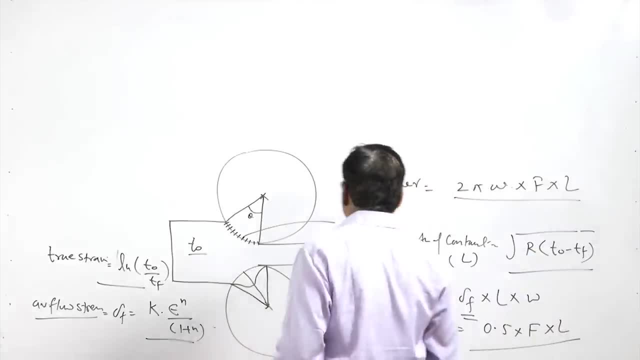 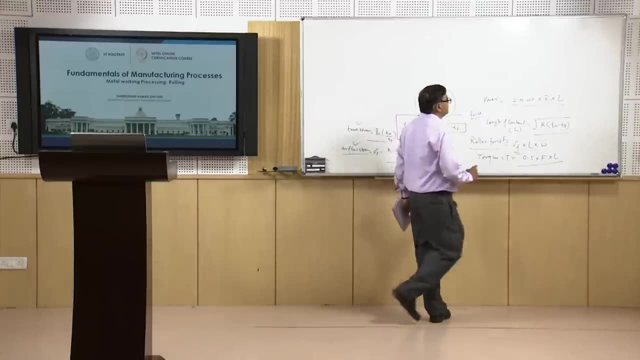 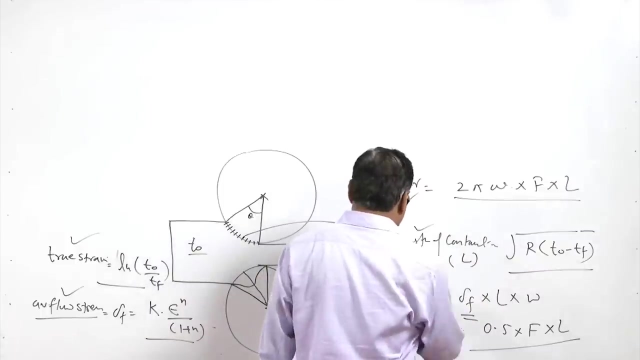 length. So these are the equations which can be used for determining the true strain, average flow, stress and the power required for the rolling, the contact length, the roll force, rolling force, the rolling force and the torque which will be acting on to the rollers. 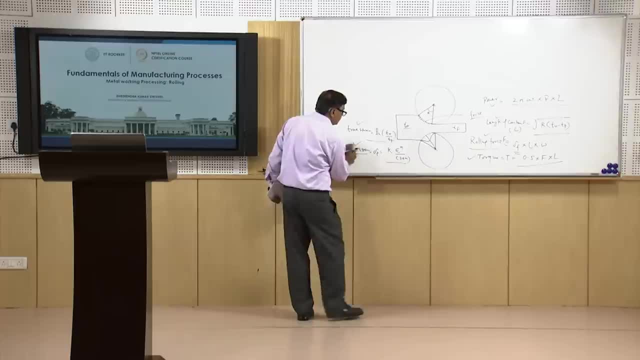 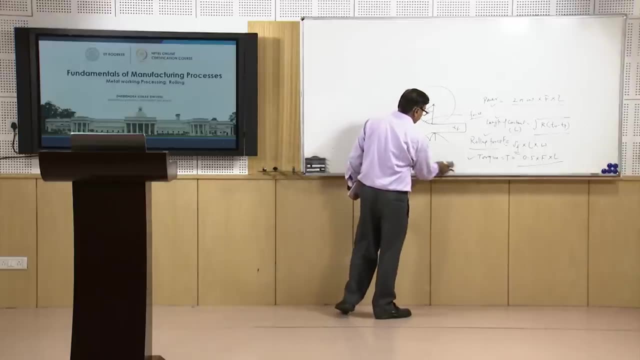 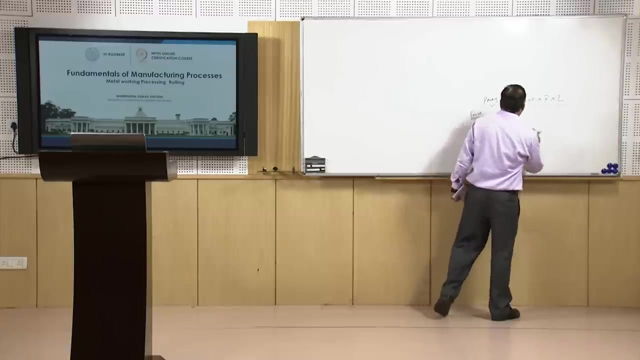 So this is So. this is how the rolling process can be analyzed with regard to the stress, strain power and the torque which will be acting on to the rollers. Now we will see. this kind of this analysis is applicable for the two roller system, but 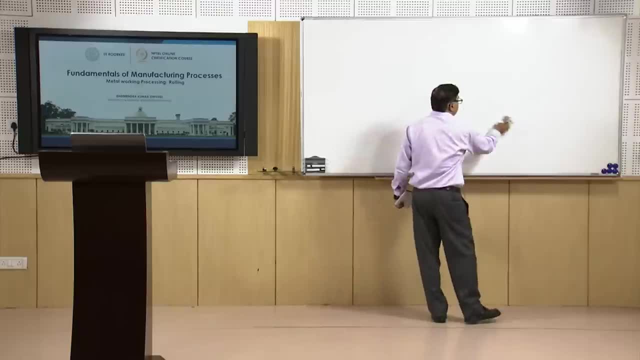 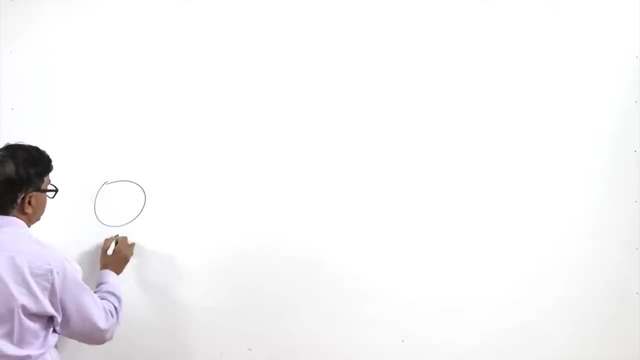 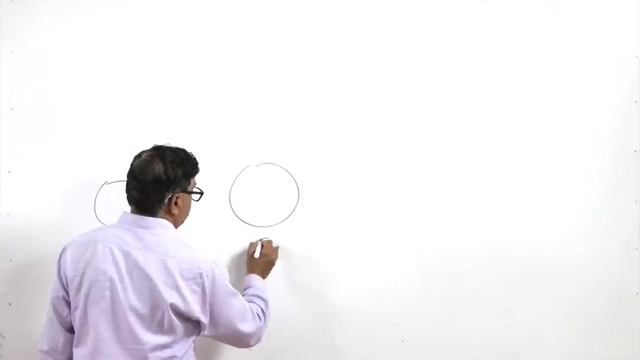 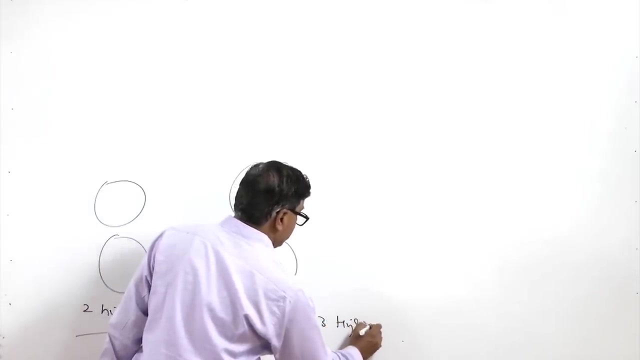 for achieving the higher draft value. So the rolling arrangements are also used. So when the two rollers like this are used, it is called two high rolling stand. When the three rollers are used like this in this case, it is called three high rolling. 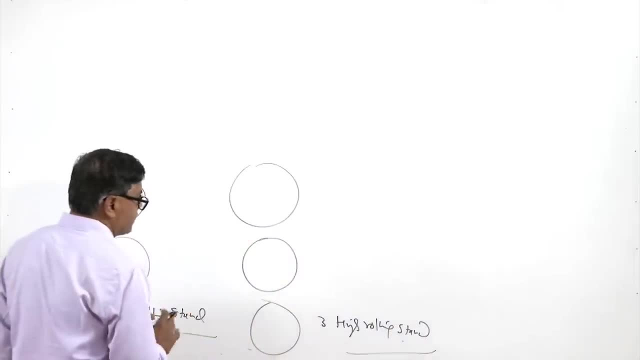 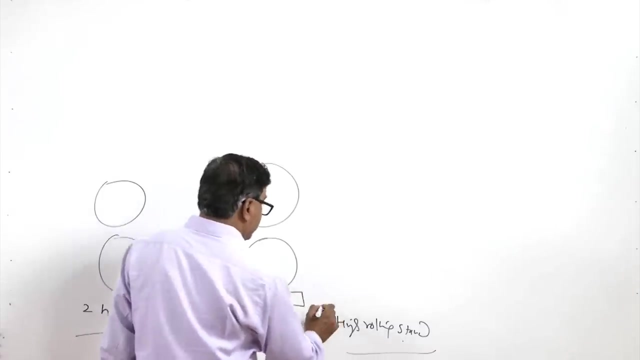 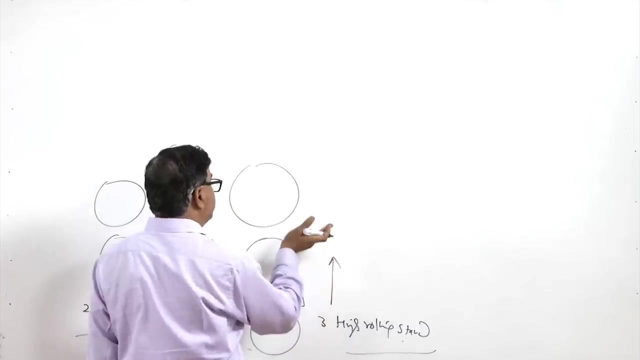 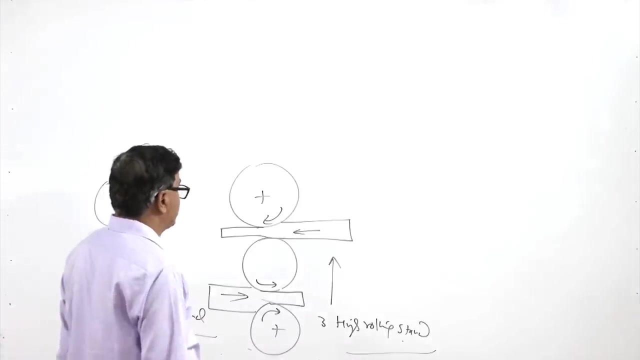 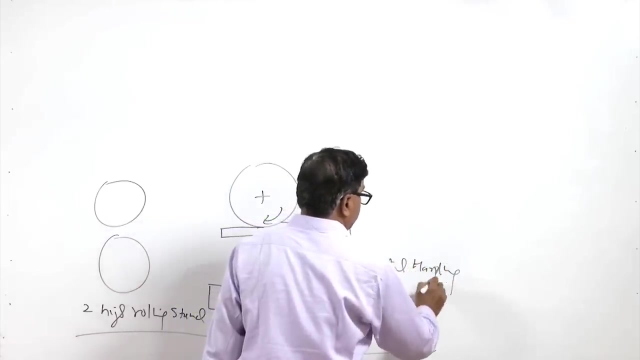 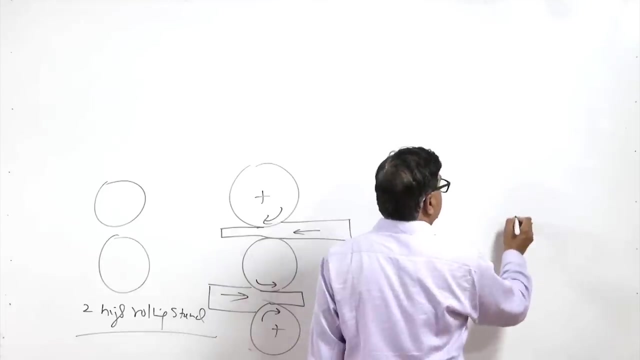 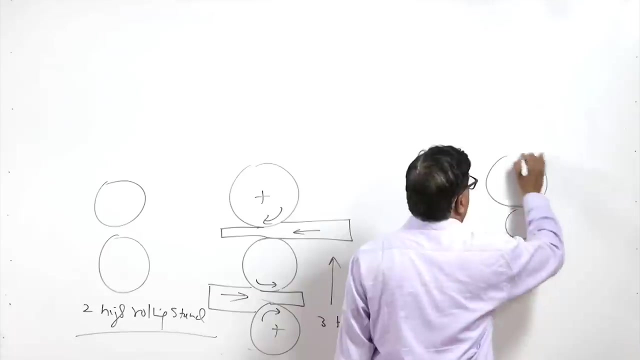 stand, And then there is a four high rolling stand. it is in this case we use the small rollers for having the higher angle of the bite, since the small rollers cannot be very rigid and strong. So, in order to provide the suitable backup, the large diameter rollers are used as a backup. 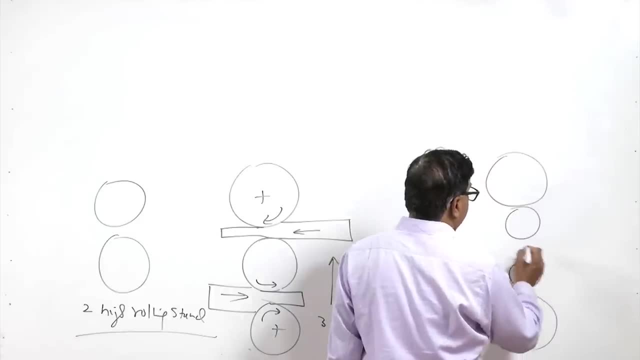 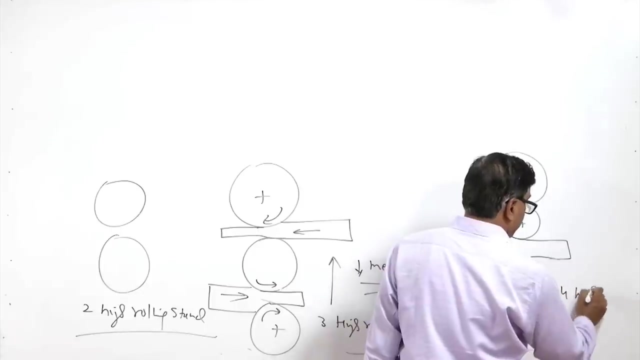 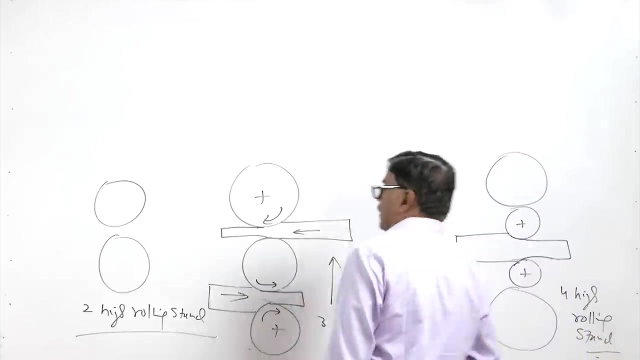 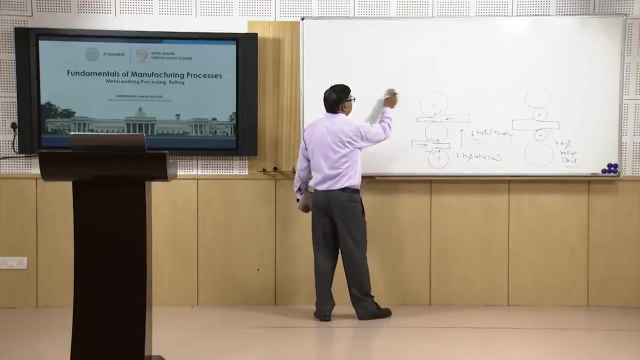 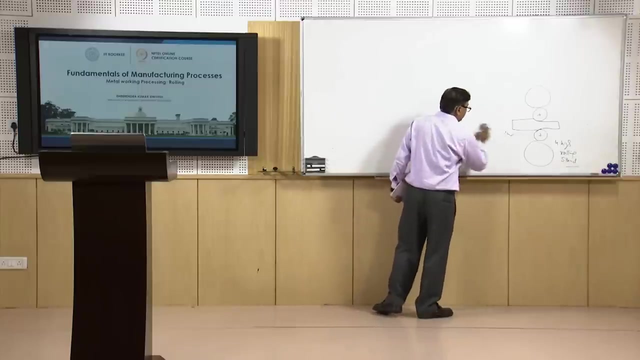 and the high angle of the bite is achieved through these. This is the arrangement for four high rolling stand. Now we also use one more arrangement which is commonly used for high draft values. That is called cluster arrangement. and in the case of the cluster arrangement again, 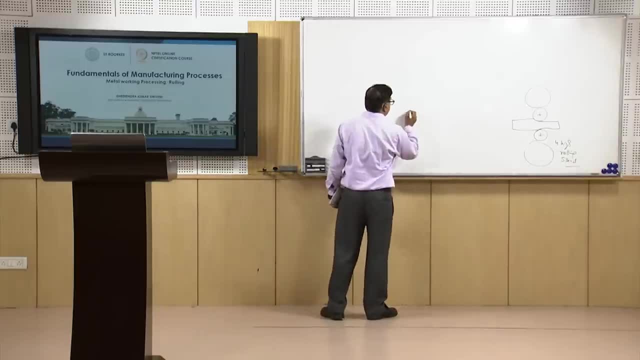 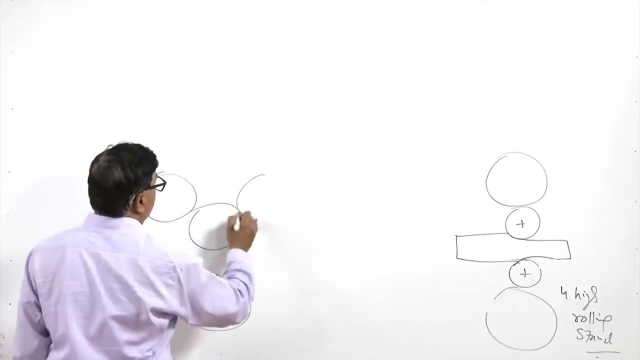 the small diameter rollers are used like this, and then these rollers are supported with the help of the four other rollers from four sides, So 1, 2, 1, 2, 3, 4.. These are the four support rollers and these are the main four working, two working rollers. 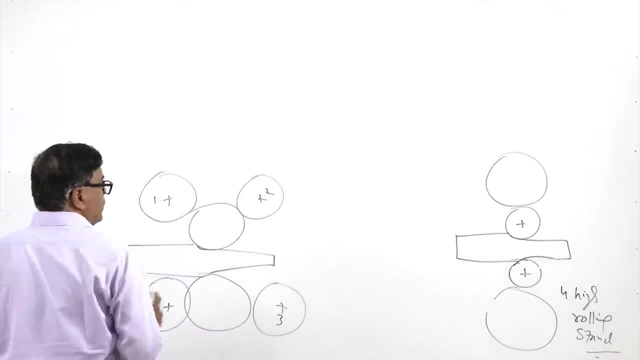 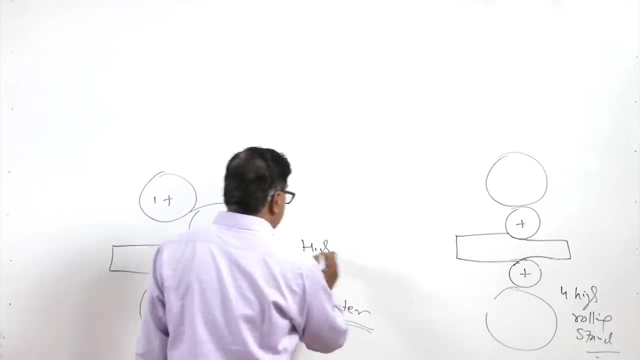 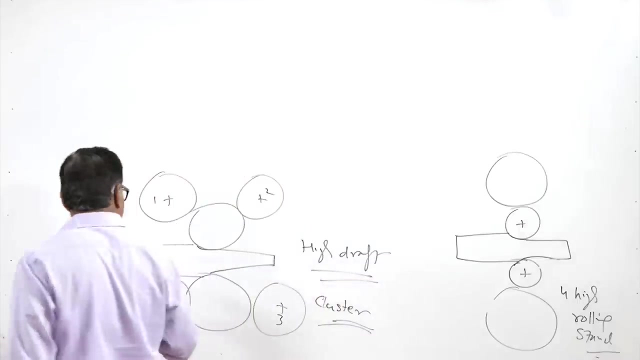 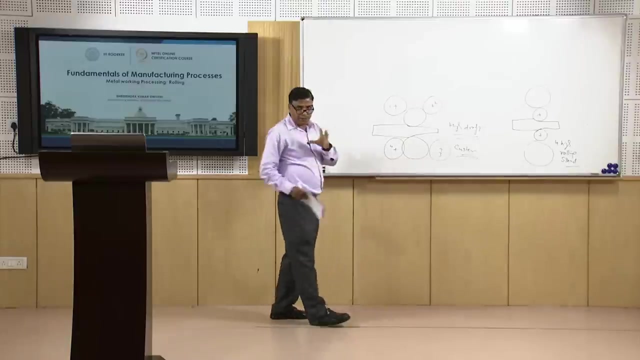 which are smaller in size. So this kind of arrangement is called cluster rolling machine and it is used for the high draft using the low small diameter rollers. The advantage of the small diameter rollers that it reduces the rolling roll separating force or the rolling force which will be acting on to the rollers. 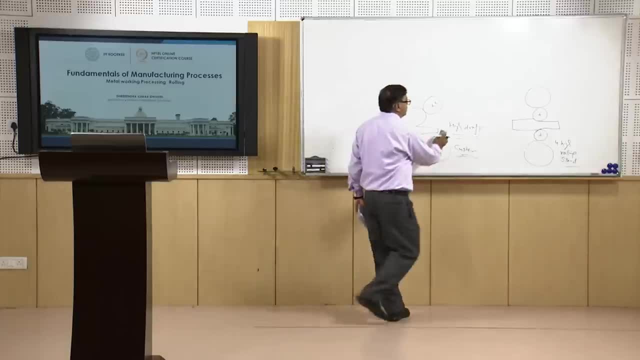 We know that when the roll, the forces act on to the rollers, then rollers tends to bend in a particular way and that leads to the non-uniform thickness of the plate which is being rolled. So normally it is expected that the rollers 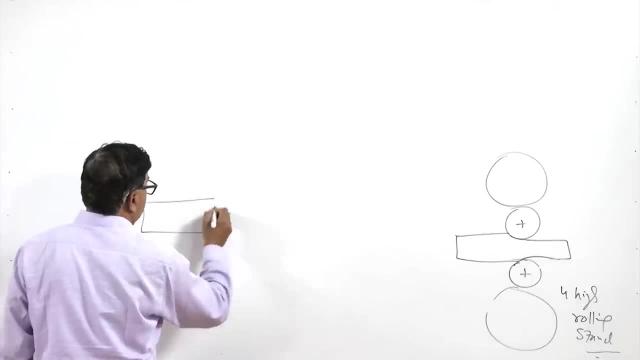 So normally it is expected that the rollers like this, these are the rollers- and between these rollers, if the plates- and they will be having the like, say, supports at the ends and the plates will be passed through these rollers like this. So because of the roll separating force, the at the centre, 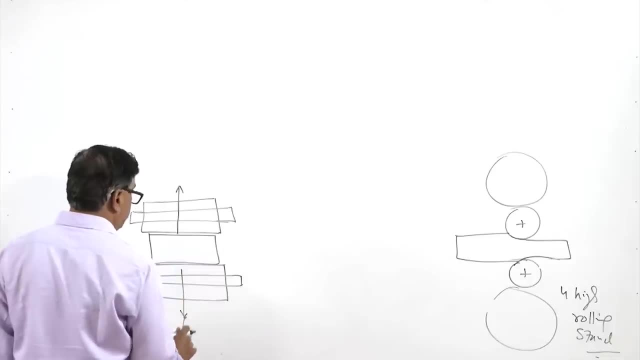 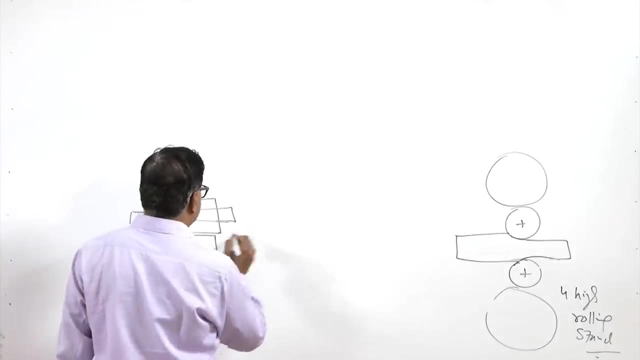 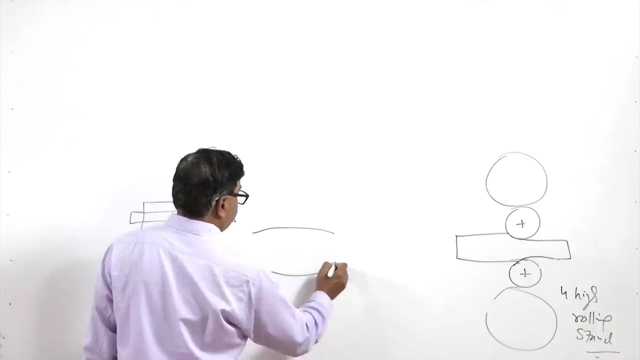 So the roll stands to bend outward and because of this outward bending of the rolls, the thickness of the plate at the centre increases like this, while at the ends it reduces. So this leads to the non-uniform thickness across the width of the plate. 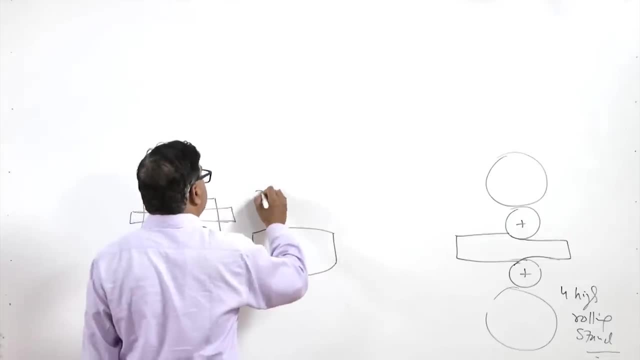 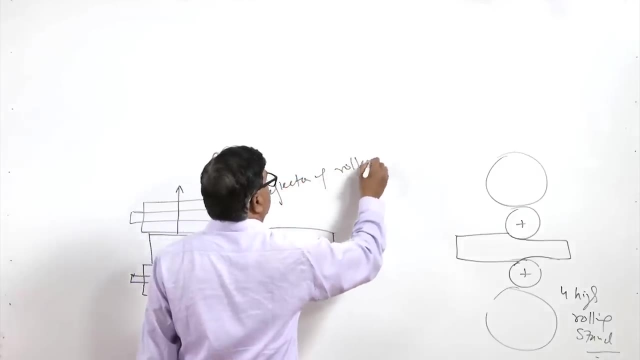 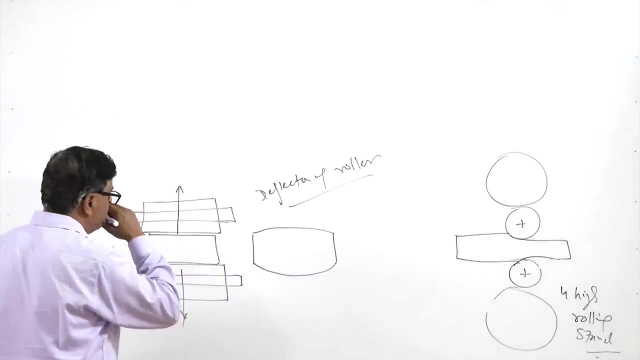 So, in order to avoid this kind of- and this is primarily due to the rolling, So this is primarily due to the deflection of the rollers, due to the roll separating force. So what is done? basically, the diameter of the rollers is not made cylindrical means. the diameter of the rollers is not made uniform, but it is slightly made of the larger diameter at the centre, So the effect or the deflection effect of the rollers can be negated. So instead of having the simple uniform diameter rollers, the diameter of the roller is slightly. 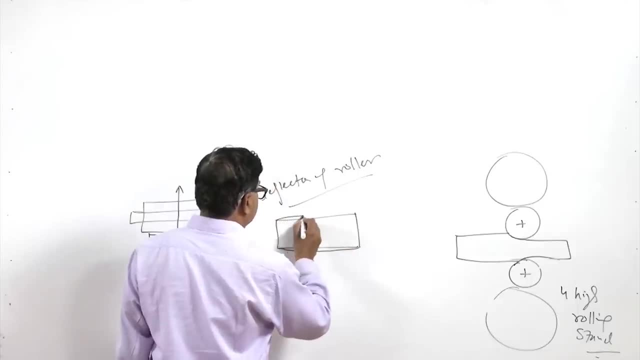 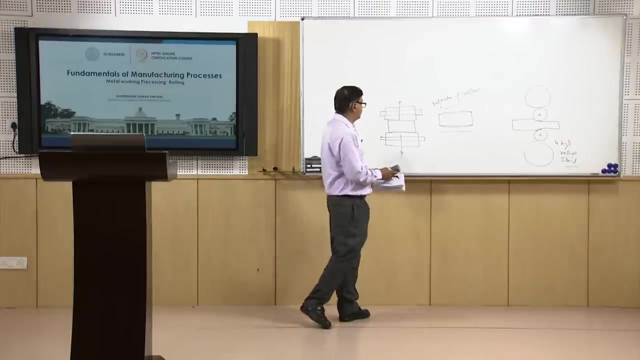 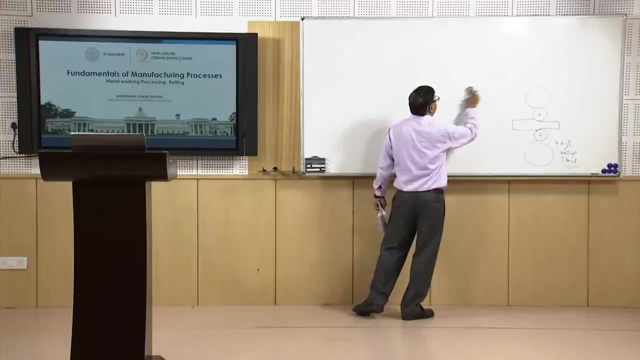 increased at the centre like this, So that even after the bending, the diameter. so when it bends the, it simply gets straightened like this and we get the uniform thickness of the rolled plates. So the bending and the deflection of the rollers which leads to the greater thickness. 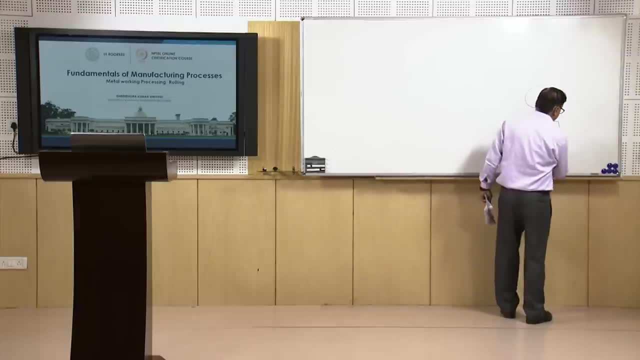 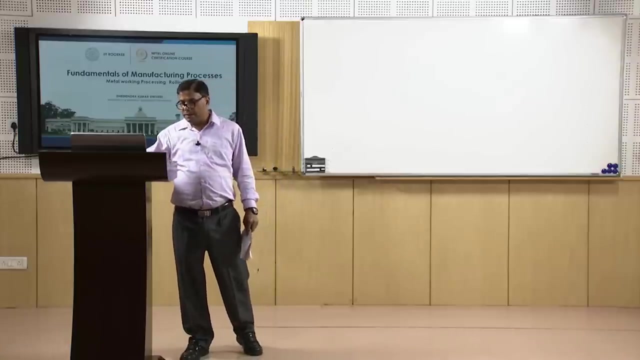 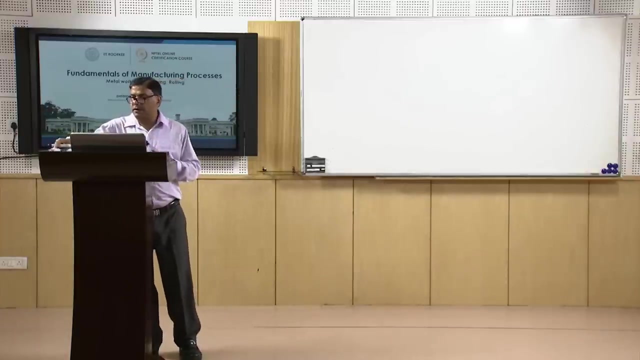 at the centre and lesser thickness at the corners. this effect can be negated or countered by making the rollers of the larger diameter at the centre and the smaller diameter at the corner. Now we will see one typical example related with the rolling strain, stress, torque and 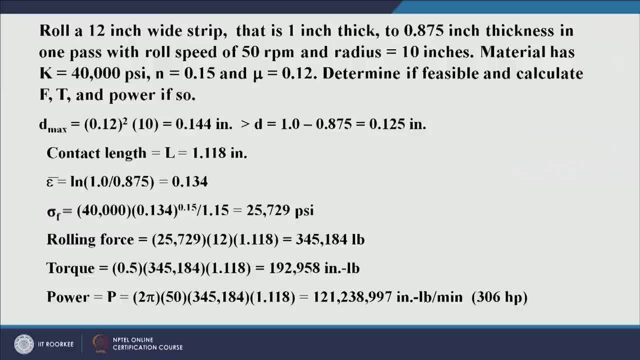 the power consumption analysis. So if we see here in this example, the rolling of the 12 inch width plate of 1 inch thickness is carried out to the thickness of 0.75 inch, So means there is a thickness reduction from 1 inch to the 0.875 inch in one pass. 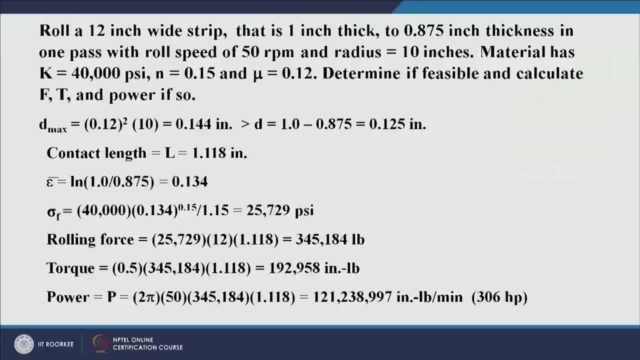 using the roller speed of the 50 rpm and the radius of the roller is 10 inches. If the materials strength coefficient K is 40000 psi and strain hardening exponent N is 0.15. And the friction coefficient is 0.12, then we have to identify whether it will be feasible. 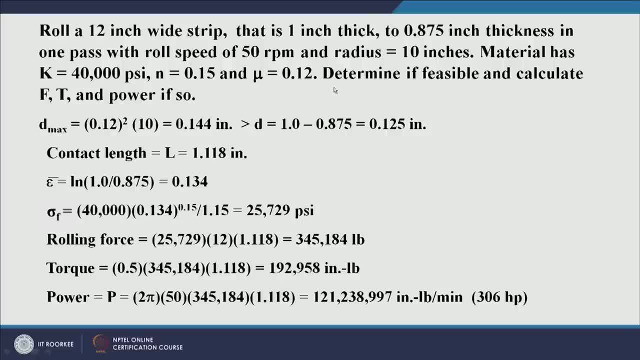 to achieve this much thickness or not, and which is normally achieved through the maximum draft value which is achievable and that we can achieve through the mu square into R. So mu in our case is 0.12.. So, since the formula for determining the maximum draft is mu square into R, so this: 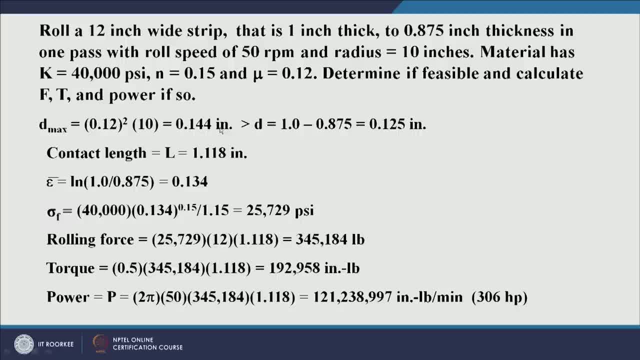 is what gives us 0.12.. So what? it suggests? that, in our case, 0.14 inch, this is the maximum draft which can be achieved, But which is much larger than what is to be achieved in our case. In this case, the reduction which is to be achieved is from 1 to 0.875.. 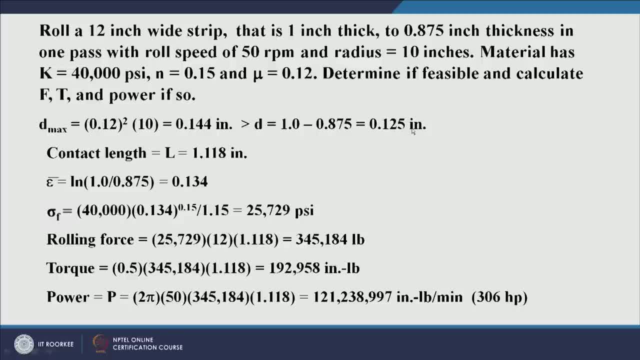 So the reduction is just up to 0.125, which is to be achieved, while the maximum achievable reduction in thickness is 0.144.. So the maximum easier to achieve this kind of the case is already feasible. I mean it is very much doable. 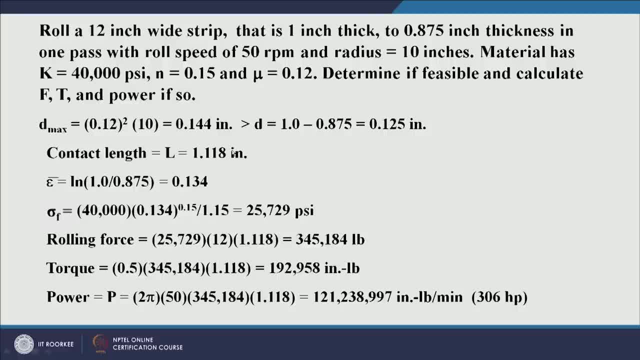 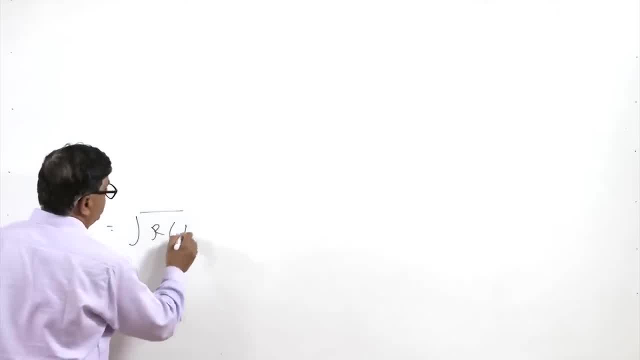 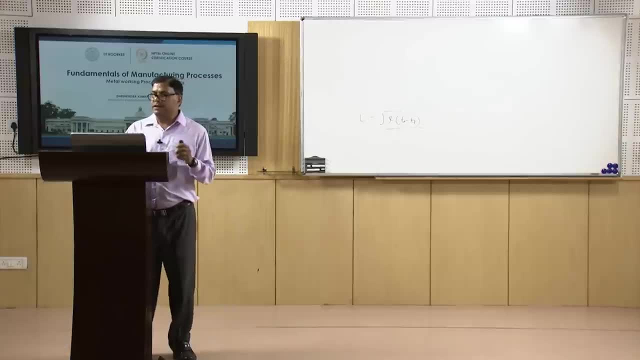 Now we can determine the contact length. The formula for contact length is already I have written. The contact length can be obtained from the square root of R, T naught minus T f. So in this case T f is the 0.875 and T naught is the 1 inch and the R is the 10 inch radius. 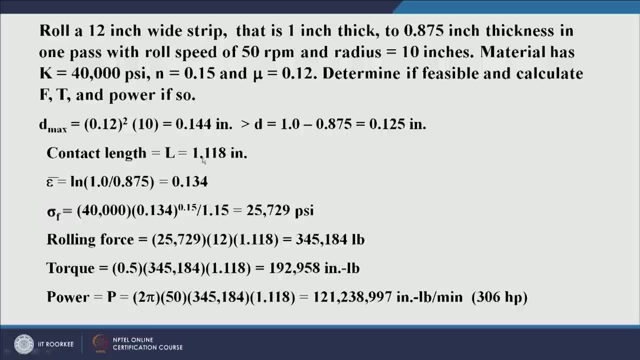 So these 3 can be used for calculating the contact length, which comes out to be 1.18 inch, and the strain which is occurring due to the rolling on account of the reduction in thickness from 1 inch to 0.875 inch. 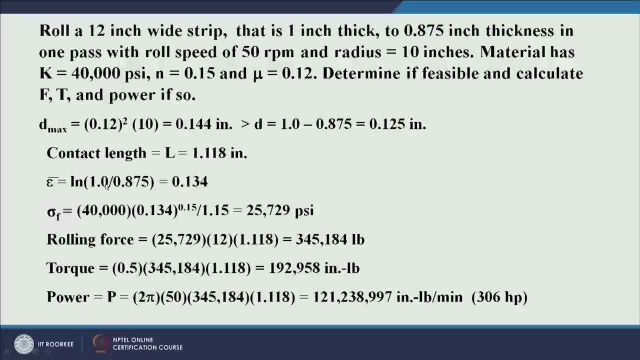 The strain can be calculated using the simple equation log of T naught divided by T f. So T naught is here is 1 inch, and T f is the 0.875 inch which leads to the strain of 0.134.. 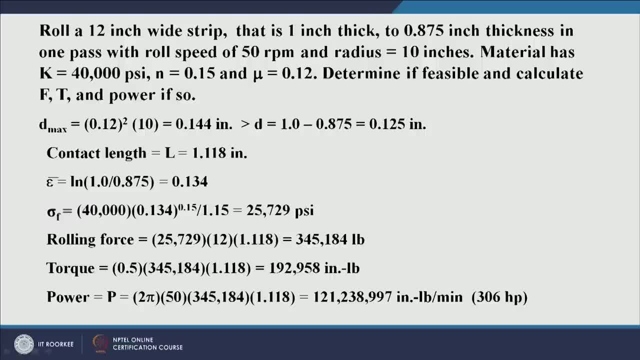 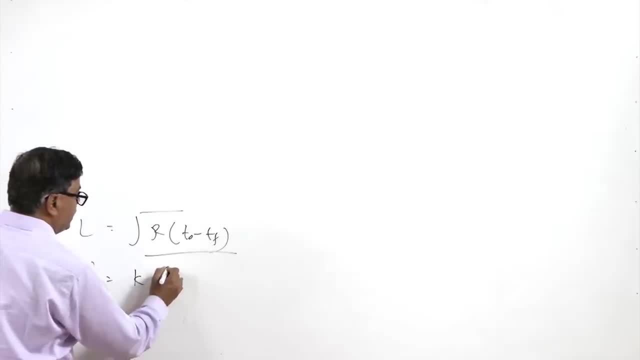 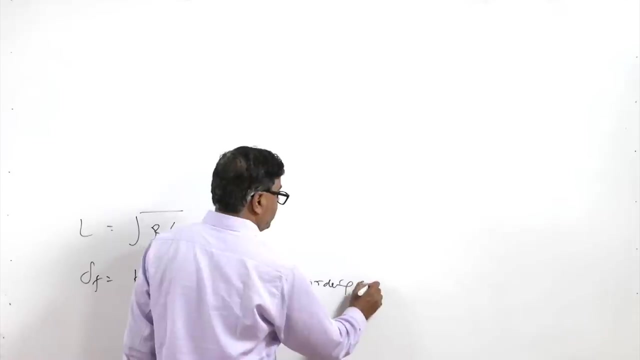 Now we can calculate the flow stress. The flow stress can be calculated using the simple equation where in the flow stress the sigma f, or can be calculated like K into the strain and raise to the power. n divide by 1 plus n, So n is the strain hardening exponent. 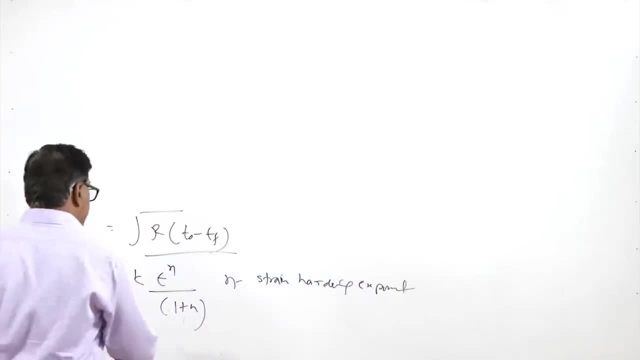 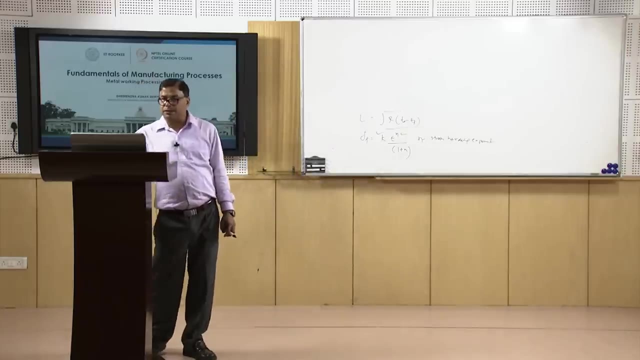 So all these values are given in our example, So here this can be used. Strain hardening exponent is here 14.5.. Strain hardening exponent is here 40,000 psi and n is 0.15 and the strain which has been 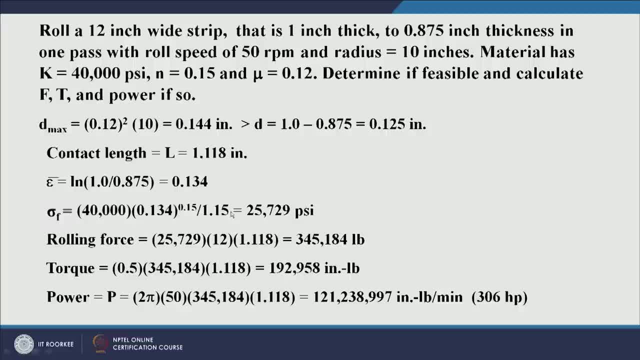 calculated is 0.134 and the n is 0.15.. So this gives us 25,729 psi. that is the flow stress. Now, using this, we can calculate the rolling force. Rolling force is the rolling force. f is obtained. 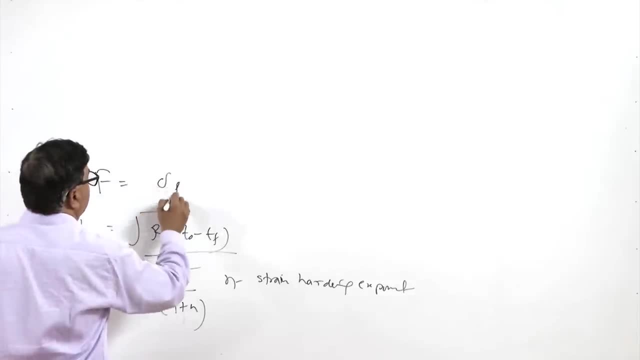 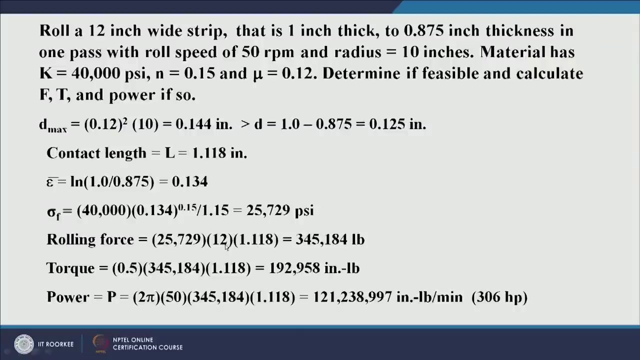 Rolling force f is obtained from the sigma f into the width and the length of the contact. So all these are there. The flow stress 25,729, 12 inches is the width of the strip and length of the contact is 1.18 inch. 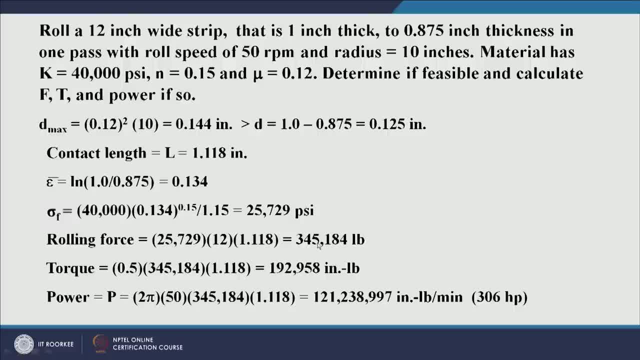 So this gives us the roll rolling force of 345184.. So this gives us the rolling force of 345184.. So this gives us the rolling force of 345184.. So this gives us the rolling force of 345184.. 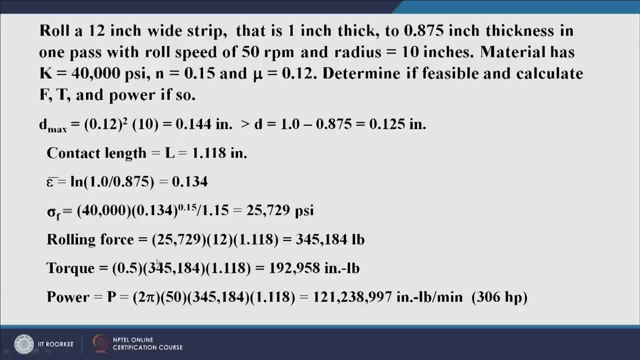 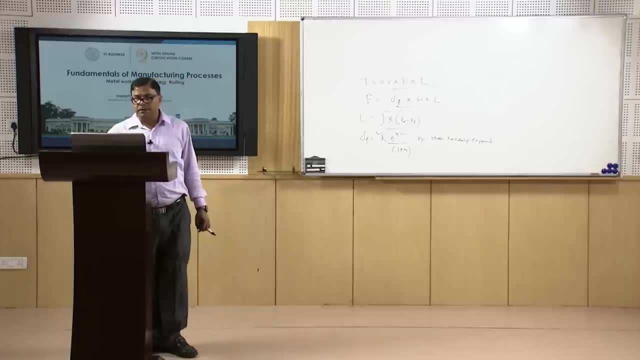 And the torque can be calculated using the formula. the torque t can be calculated 0.5 multiplied by f, the rolling force multiplied by the contact length. So in our equation here, 0.5 multiplied by the rolling force is 345184 multiplied by. 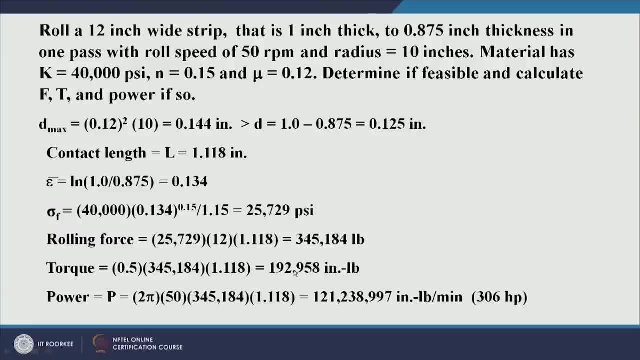 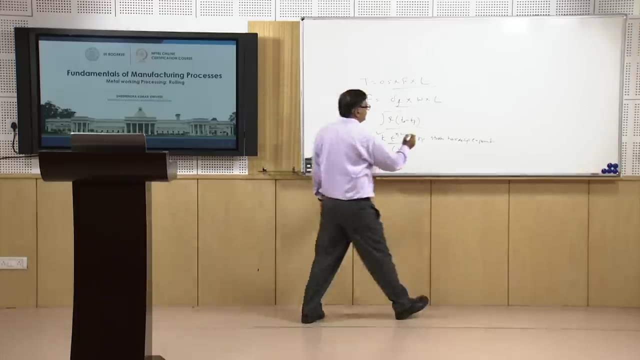 1.118. that is the contact length. So this gives us 192958 inch pond And the power consumption for the rolling, for reducing the thickness from 1 inch to 0.875 inch, can be calculated using the simple equation. as I have mentioned, that power consumption. 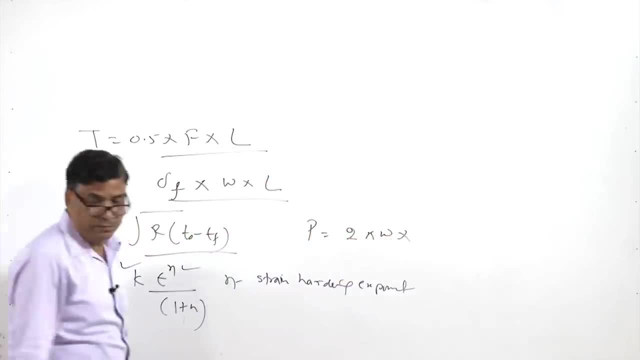 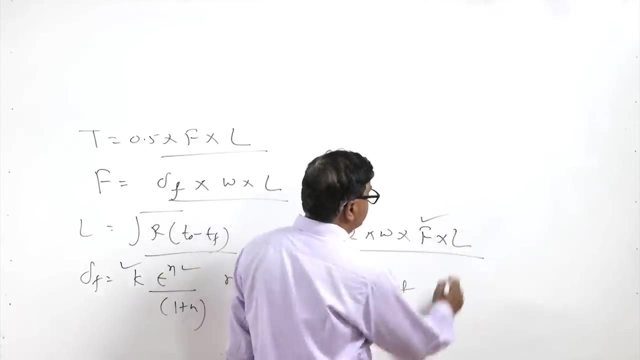 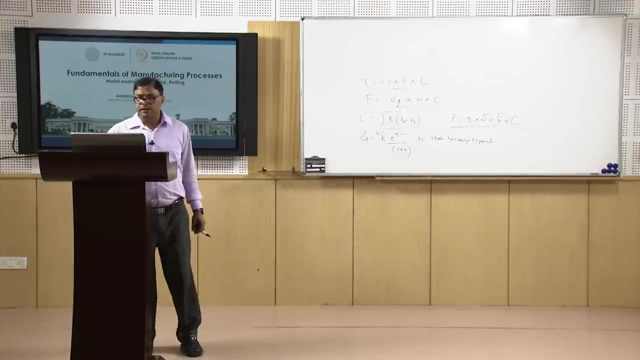 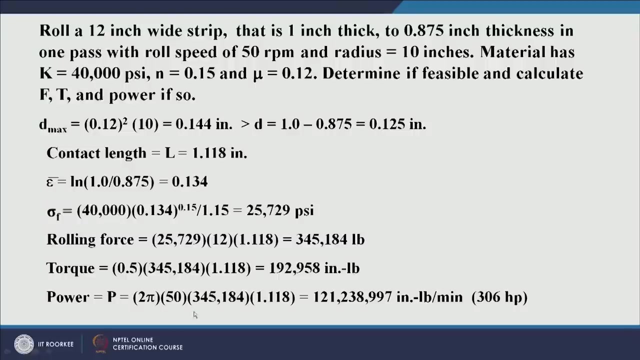 is from the 2 pi omega into the force, into the contact length. So this is the rolling force, L is the contact length, omega is the rotational speed. So using these three terms, the power consumption can be calculated using 2 pi. 50 is the rotational. 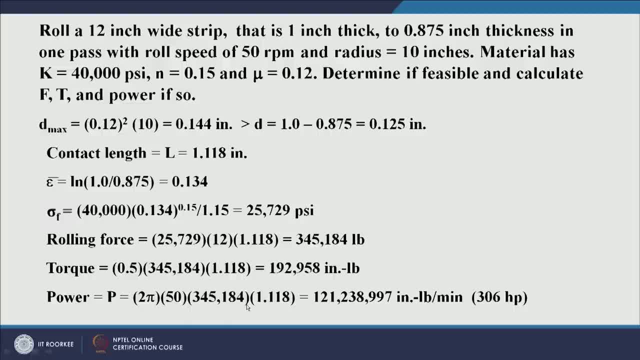 speed omega and the 245. 184 is the rolling force and the contact length is 1.18.. This gives us 121, 328 and 997.. Inch bond per minute, which is corresponding to 304 HP, is the power required. So now I will summarize this presentation. 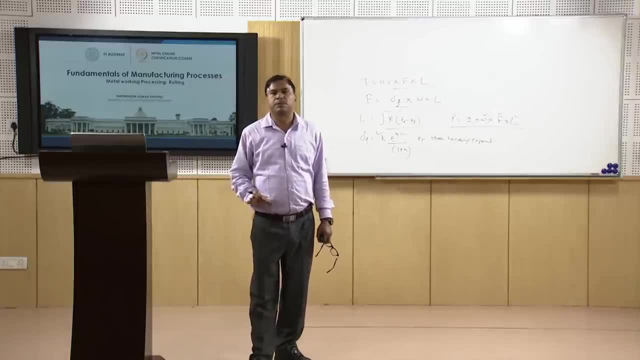 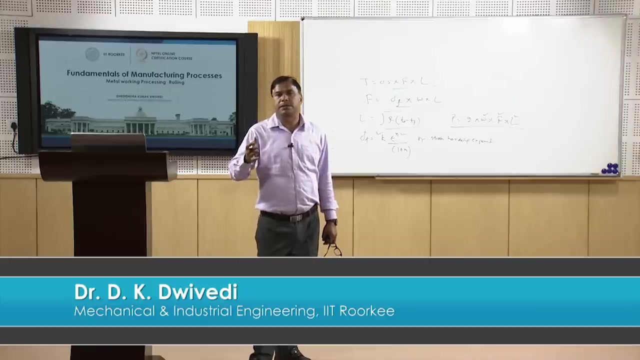 In this presentation I have talked about the rolling process, which is primarily used for reducing the cross section, and the reduction in cross section is primarily used by reducing thickness and increasing the length, while the rolling produces the components of the uniform cross section along the length.